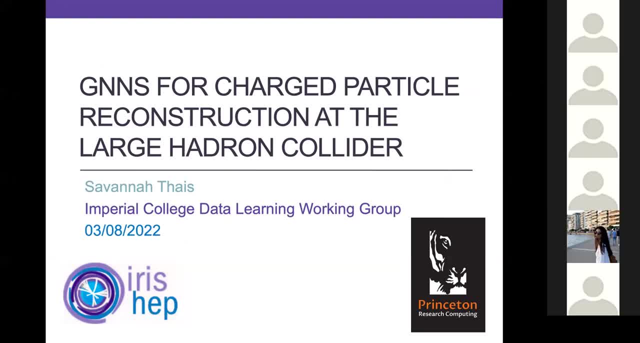 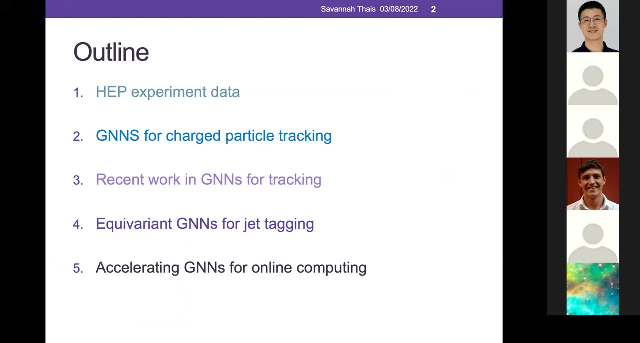 working at the intersection of physics and engineering. I'm a research scientist at physics and machine learning, So I'm going to be talking about particularly using graph neural networks for charged particle reconstruction at the Large Hadron Collider- Great. So a quick outline. I'm going to talk about kind of what data looks like coming out of high. 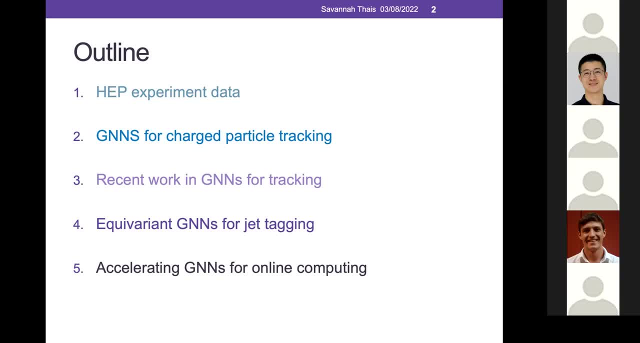 energy physics experiments. Then I'll talk about work on using what graph neural networks are and how we can use them to do research. Then I'll talk about some of the really interesting current work that my group has been doing on this topic. Then I'll introduce another new paper that we just put out on a slightly 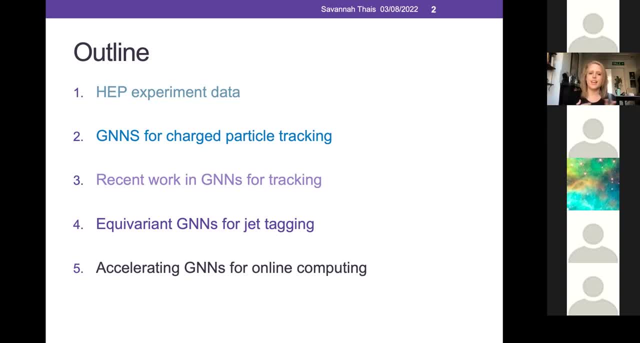 different reconstruction task, but still using GNNs. And then, if there's time, I'll talk a bit about how we can accelerate the inference of these GNN algorithms. Cool, So, starting off with a very simple graph neural network, I'm going to start with this graph neural model. 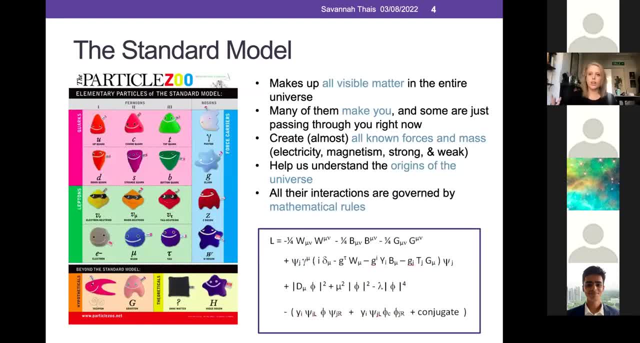 high energy physics data. So in particle physics we have this model, called the standard model, that describes the particles that make up all visible matter in the universe, including, you know, us humans, all of the matter on Earth in the universe, including light and other particles. 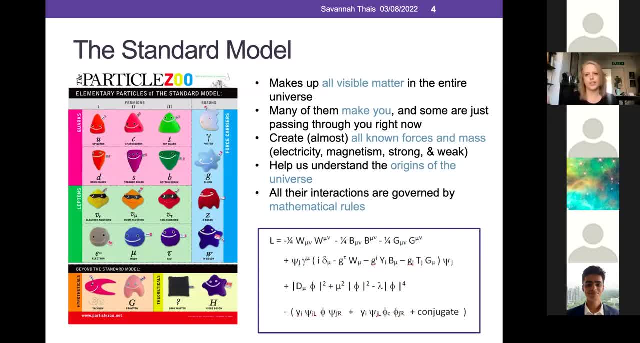 that we're maybe not as familiar with, that are like passing through us right now, that are produced from different reactions and interactions of particles, And the standard model also describes the particles that create almost all of the known forces in the universe of things like electricity. 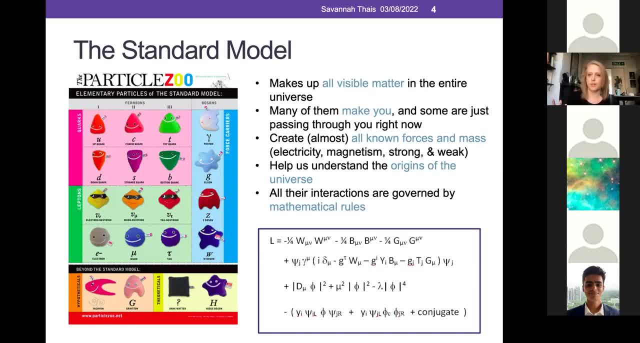 and magnetism, the strong force that holds quarks together inside of protons and neutrons, the weak force that governs decay, decays of charged particles, And so there's a really, really awesome model that has helped us understand a lot about the origins of the universe. 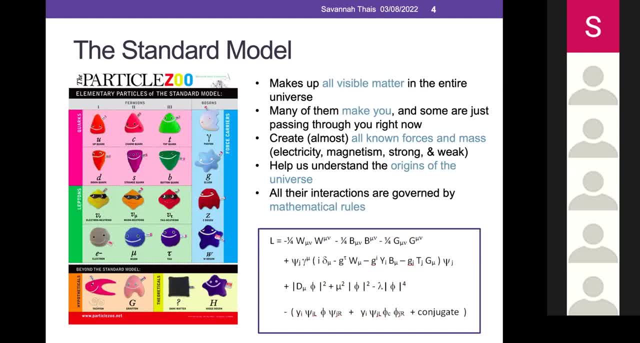 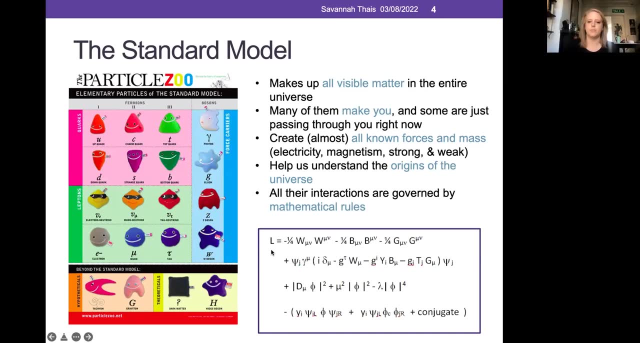 the way that different particles interact with each other to form matter and different types of materials, And this model and the interactions of all the different particles included in it are governed by this set of mathematical rules described by the standard model Lagrangian, which you can see a reduced form of here. So this is a really, really powerful model. 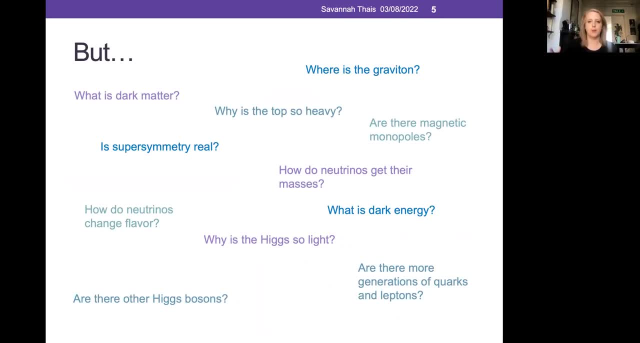 But it doesn't answer everything about particle physics. There are a lot of outstanding questions that we're still interested in in studying. So in particular, I said the standard model describes almost all forces in the universe, So it actually does not describe gravity, which is kind of the 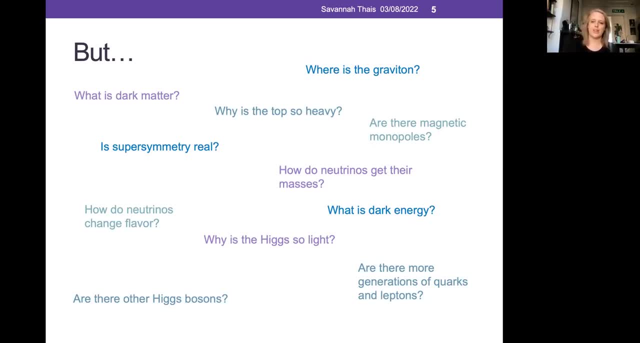 most intuitive force that we're all aware of and interact with, on you know constantly, And so there's actually no quantum model of gravity right now that has been verified experimentally, So that's a big gap in the standard model. There's also lots of other questions. 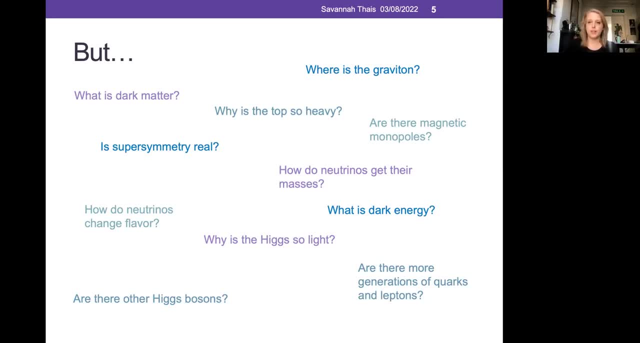 some of which I've highlighted here. For instance, dark matter is a big, open area of research. We know that it should exist, but we don't know what the particle nature of dark matter could be. And then there's lots of other kinds of theorized particles. 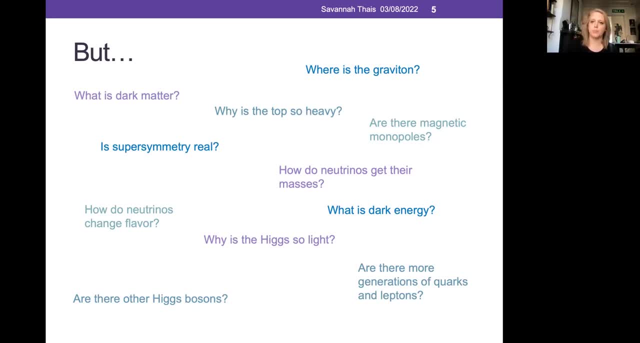 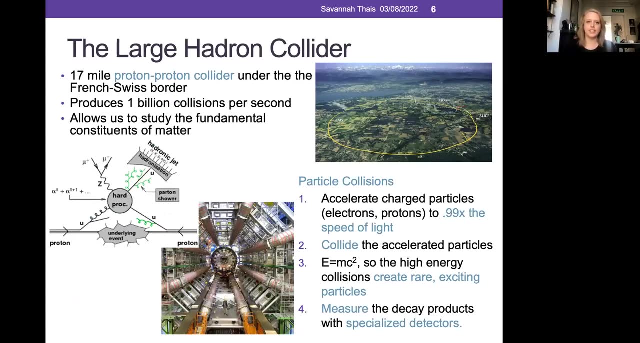 that could answer some questions that are left open by the standard model. So, in order to try to answer some of these questions that I just highlighted and to look for new types of particles that people have theorized, we have this incredible machine: the Large Hadron Collider. 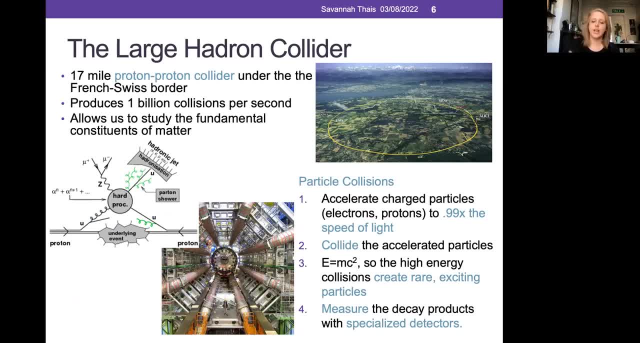 which is a 17 mile proton-proton collider ring under the French-Swiss border that collides billions of protons per second, at almost the speed of light, And because we have this mass-energy equivalence described by E equals MC, squared, these really high collisions, high-energy collisions. 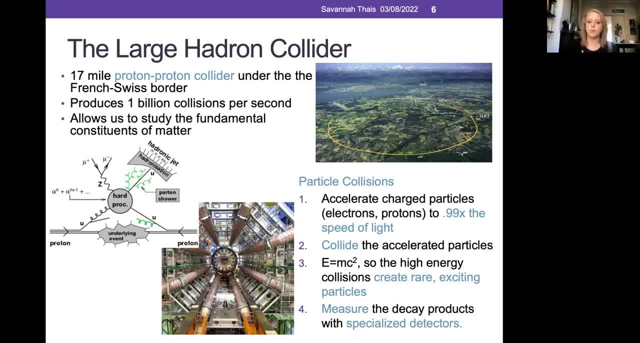 can create new types of particles, including really heavy particles, very rare particles that don't normally exist on Earth, And then we can measure the decay products of these particles with specialized detectors and we can capture really rich, multi-dimensional, complex data. 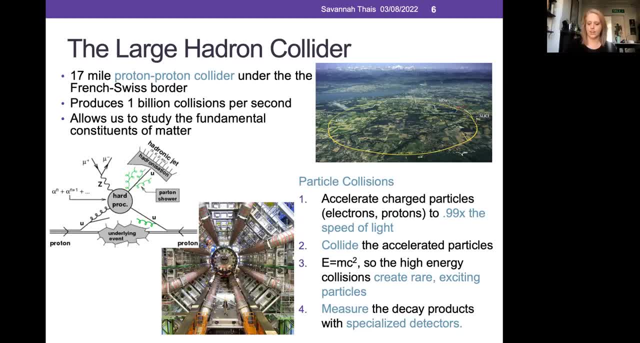 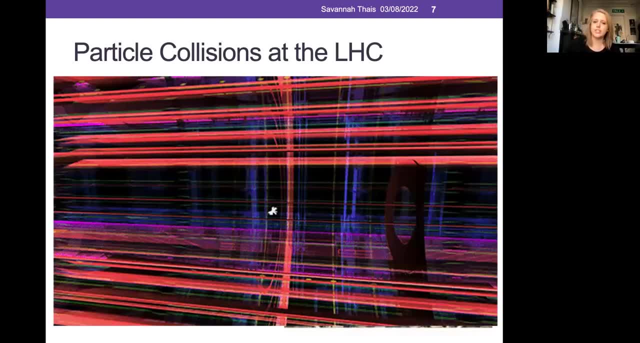 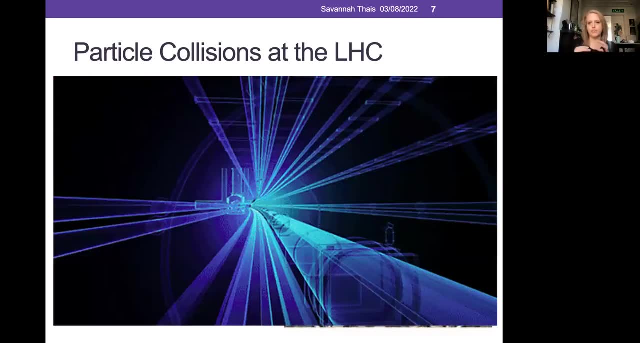 And then we can use these data sets about these particle decays and interactions. So here's one of my favorite- just little visualizations of kind of what happens inside the LHC. So you see, we have protons coming in from both sides. They collide with each other inside this really. 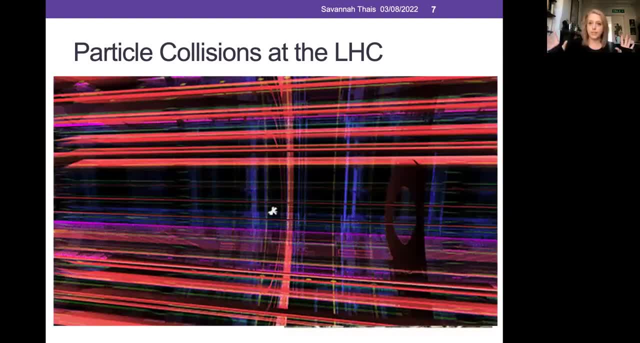 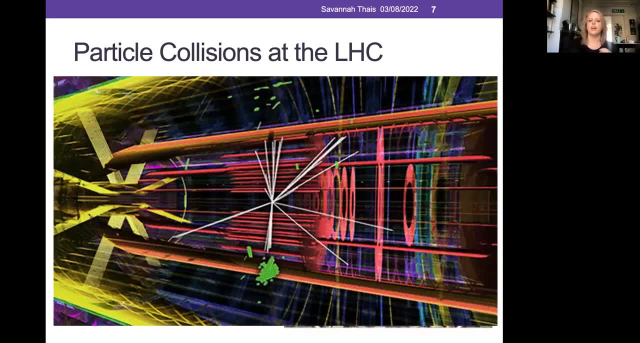 multifaceted, multi-layer detector and they create sprays of new particles And our goal is to, on the side of this, on the software side of this work, is to take the readouts of the detector, information about how those new particles interacted. 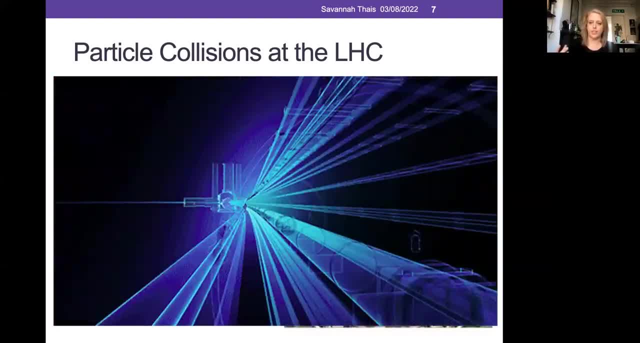 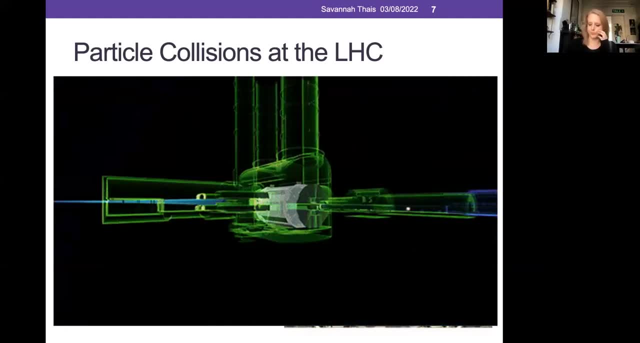 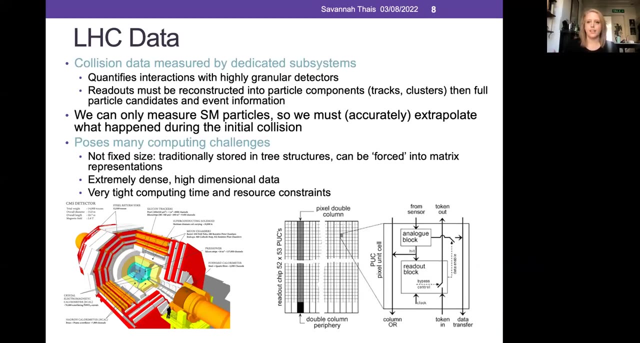 with the material of the detector and use software and data processing and machine learning to figure out what actually happened right at that collision point. So, like I mentioned, the data from these collisions is measured by detectors with dedicated subsystems And so when the particles are created and they move outwards, 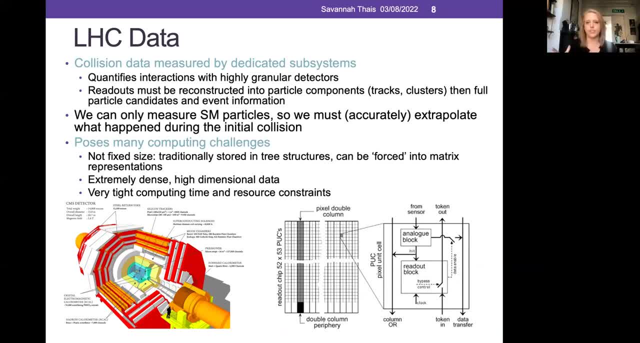 from that interaction point. they interact with different types of material in the detector and they deposit different amounts of energy in the different components. Then that energy is read out with electronics and those readouts have to be reconstructed into particle components like trajectories and energy deposit. 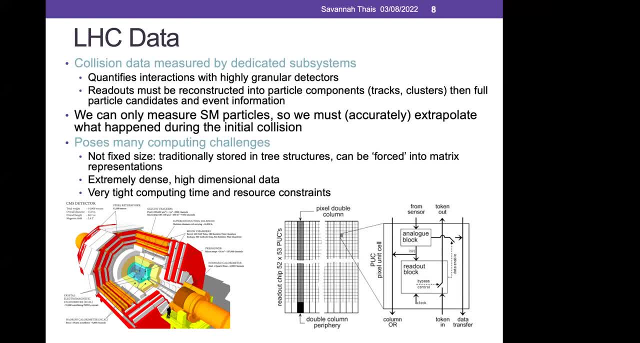 groups And then those are further reconstructed into energy, to particle candidates. so we can try to figure out. there was a muon here, there was this kind of quark here. they came from the same interaction or a different interaction and we can start to. 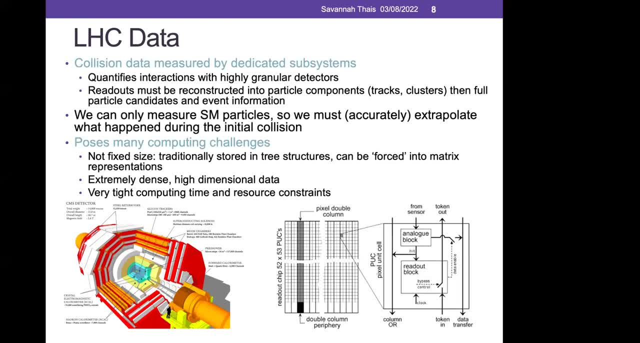 reconstruct the full physics picture of what happened at that proton-proton collision. There's a lot of difficulties with this kind of reconstruction. In particular, we can only measure particles that exist in the standard model and ones that interact with matter. So there's lots. 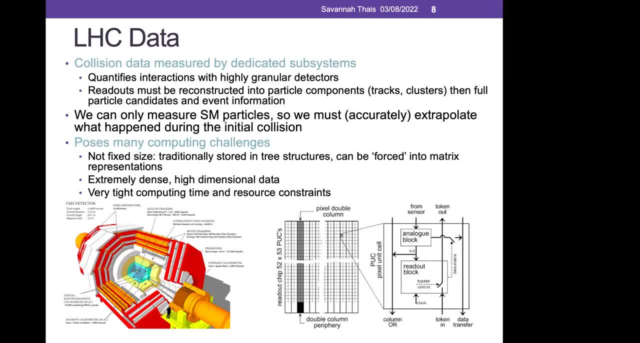 of particles that could be created that we can't necessarily measure. so it's really important that our reconstruction and data processing is very accurate, because we have to do things like see if there's missing energy from the event, If not all of the energy from the original collision is. 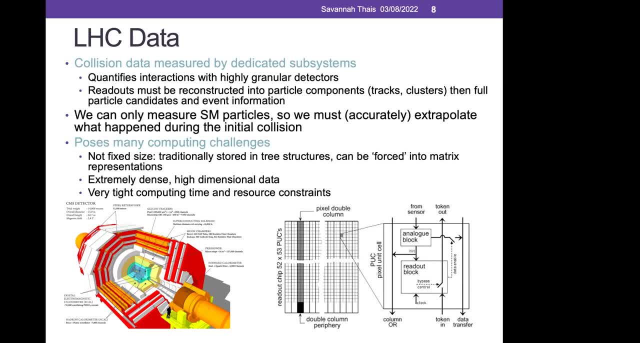 accounted for. then we can extrapolate that there were other particles there that we're not able to measure And things like that. so it's very important to be hyper accurate in this type of reconstruction. But there are several challenges with that, in particular for kind of traditional data formats. 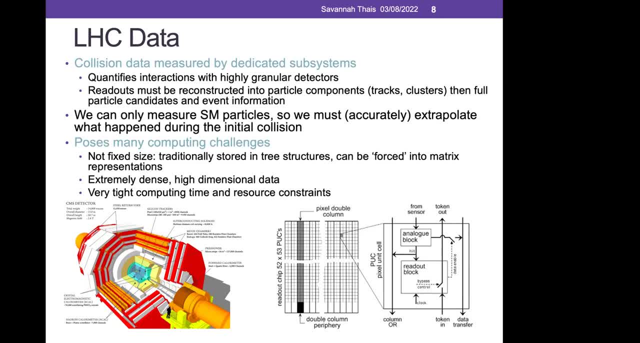 that we use in machine learning. So one challenge is that the data is not fixed size. We don't know how many particles are going to be created in any collision. We don't know what their decays are going to look like, so it's hard to be. 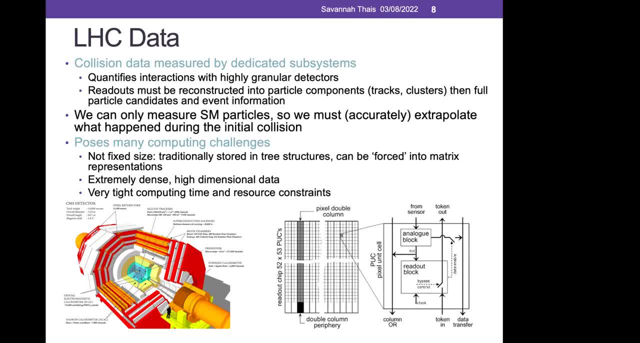 sure, In the past we have tried to force this into kind of grid-like representations like we typically use in just standard neural networks, or even images like we use in convolutional neural networks. but that always involves either some amount of padding or information loss. 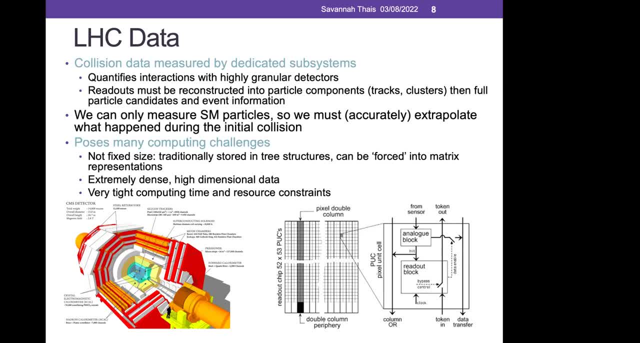 Another issue is that the data can be very dense and very high dimensional, so it can be difficult to think about good data structures to represent that. And then a really big constraint for building these data processing algorithms is that we have extremely tight computing time and resource constraints. I mentioned we are colliding billions of protons. 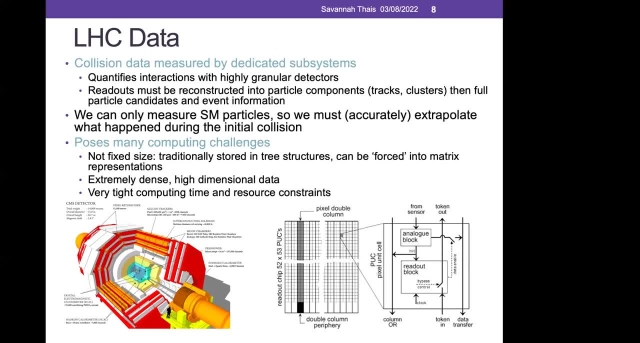 a second. That creates way more data than we can actually store for further processing. so we have to have very, very efficient online data processing algorithms that work on the order of a few nanoseconds to decide if data is valuable to store or not, And this can be. 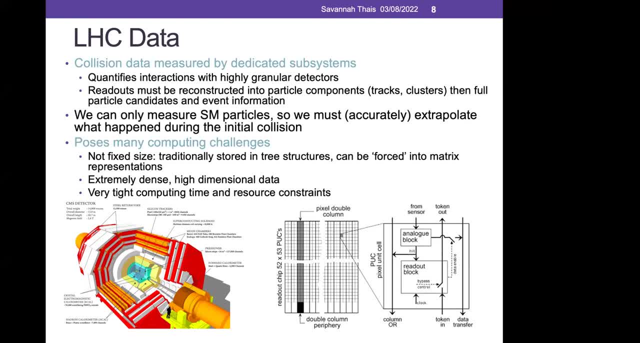 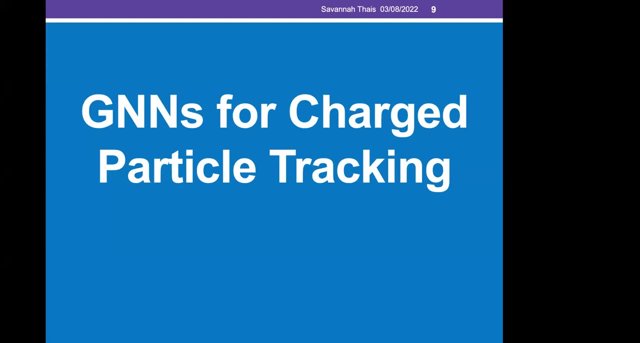 very high stakes. Some of the processes we're looking for happen once in a trillion collisions, so we want to be really careful that we're not throwing away important information. Okay, so now I'm going to talk about a specific kind of task in that data reconstruction scheme. 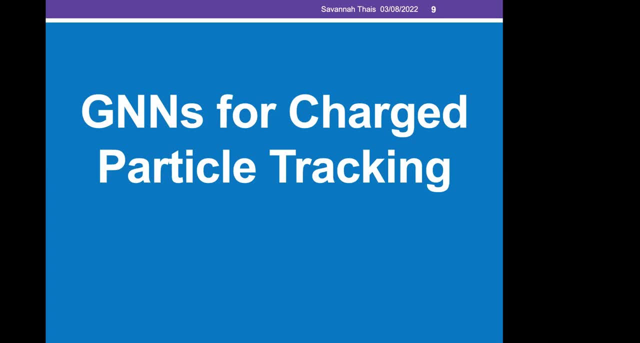 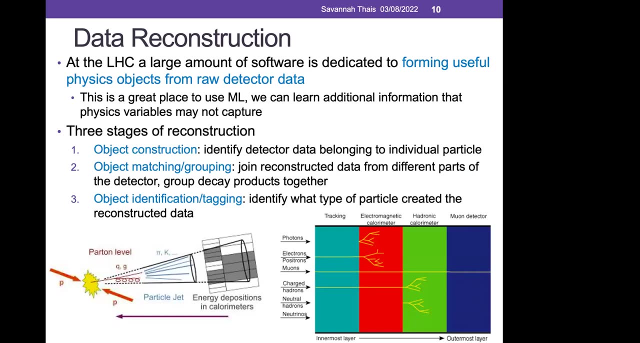 that I mentioned called particle tracking. So, like I mentioned, there's a large amount dedicated software for forming physics objects from that raw detector data. This is a really great place to use machine learning, because traditional approaches before we really started incorporating machine learning in particle physics research was based a lot on kind of derived. 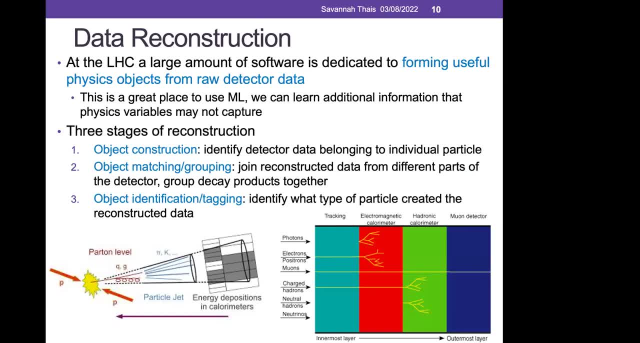 physics-based variables that created information loss. But machine learning, which is designed often to look to work on high dimensional data sets, can help us avoid some of that information loss and we can actually go right from the detector readouts and use those directly in machine learning algorithms. 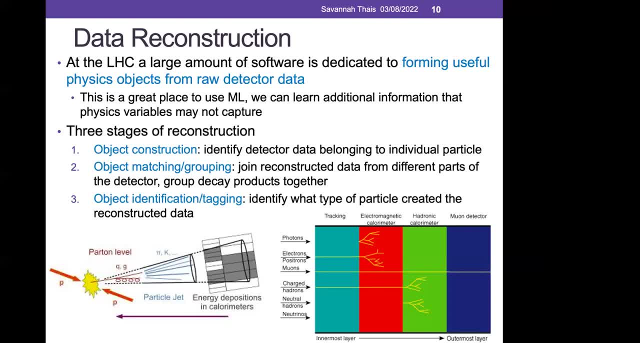 So there's kind of three main stages of data reconstruction. So there's object construction, where we take the raw detector data and we try to identify which components of it belong to individual particles. Then there's object matching and grouping, where so we try to match, we've identified objects in the different components. 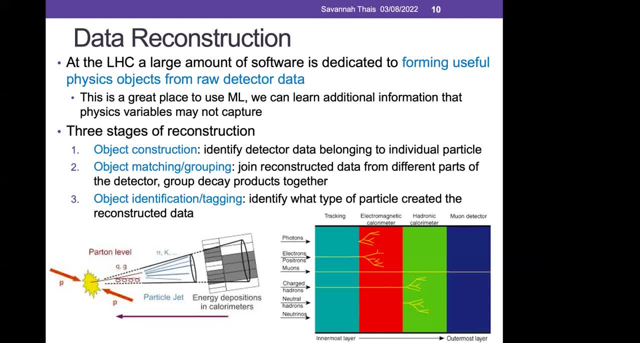 of the detector that belong to a single particle, Then we try to join those together and so that we have all the pieces of an individual particle grouped together. We also try to group things- decay products- from a single particle that maybe decayed while it. 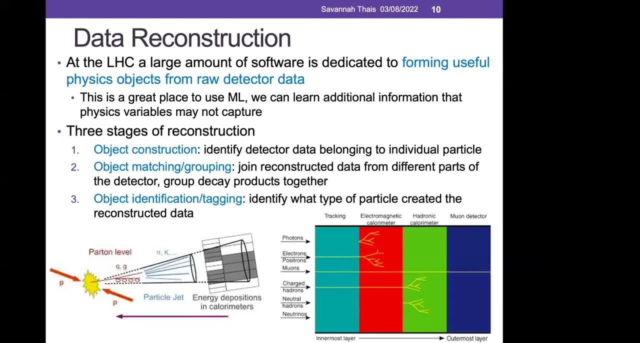 was in the detector. We try to group all of those components together as well. And then there's object identification, or sometimes we call it tagging, where, okay, now we have all of the information, or we think we have all the information from a certain particle in the detector. So can we? 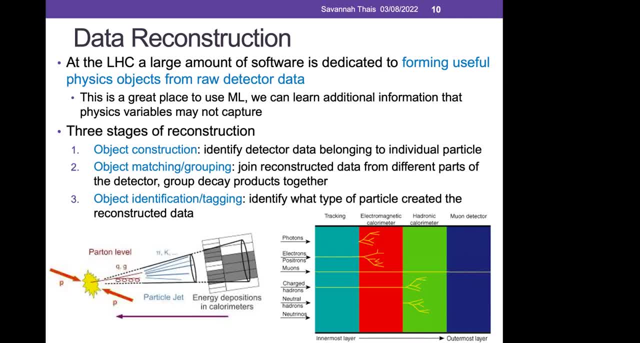 identify then what type of particle that was based on, how it moved, what its charge was, maybe how it decayed. So I'm going to focus on particle tracking, which is a task in that first set of object construction. So I'm going to focus on particle tracking, which is a task in that first set of object construction. 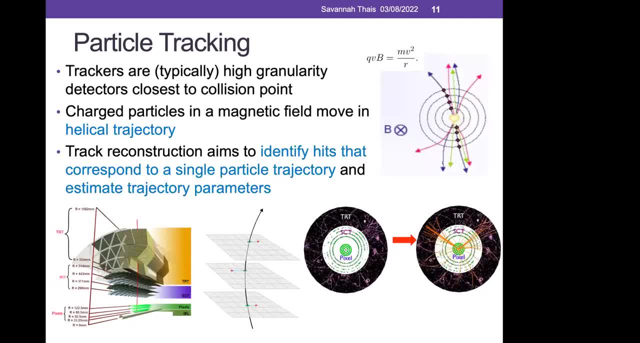 So I'm going to focus on particle tracking, which is a task in that first set of object construction. So this deals with data from what we call the tracker, which is typically a very high granularity detector that's closest to that proton-proton collision, So we get very high granularity. 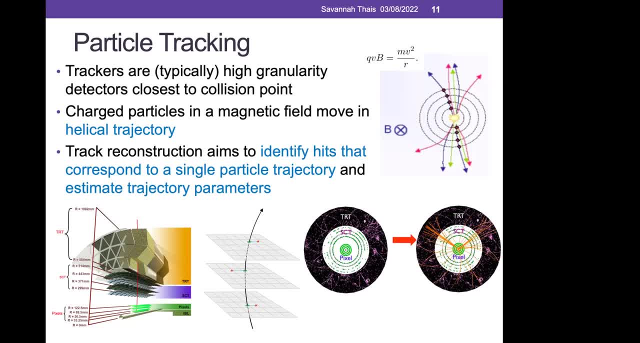 information about how a particle moved out from the collision point towards the outside of the detector And in particular charged particles, which is primarily what we can measure at these detectors in a magnetic field. So the whole detector is set inside a very, very strong magnetic field. Those charged particles move in helical trajectories. 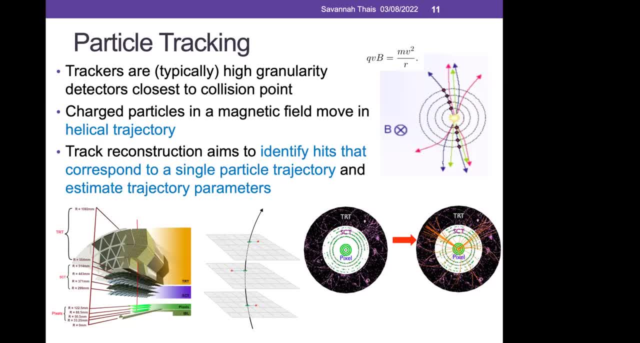 because they're curved by the magnetic field, And so track reconstruction tries to take basically a point cloud of how all of the particles that were produced in a single collision have moved out through that high granularity field, and then we can measure how they moved out through that high granularity field. 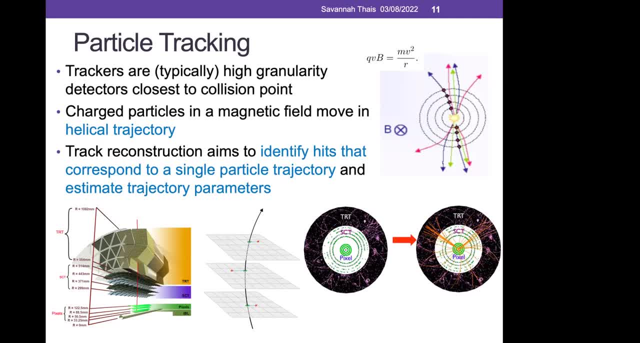 And so track reconstruction tries to take basically a point cloud of how all of the particles that were produced in a single collision have moved out through that high granularity field. It takes that point cloud and tries to identify individual particle trajectories from that point cloud and then estimate the different parameters of those trajectories. So 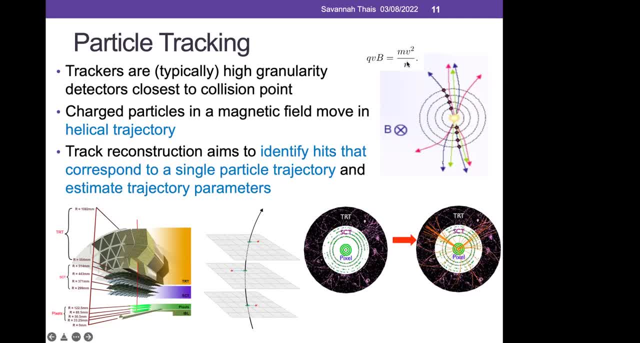 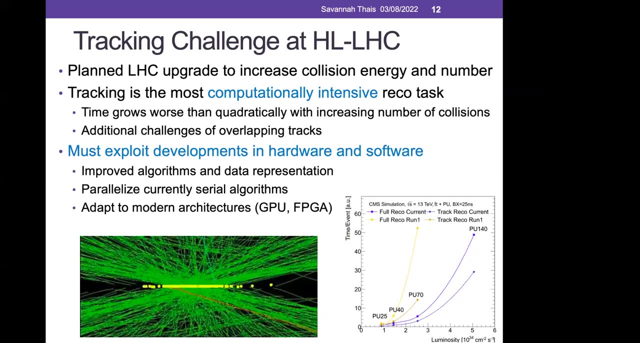 we try to get the radius of the track, which we can then use to get the velocity of the particle and therefore its momentum. So this is a really important step in doing any kind of physics work with the data that we get out of these detectors. Like I said, it's one of the first. 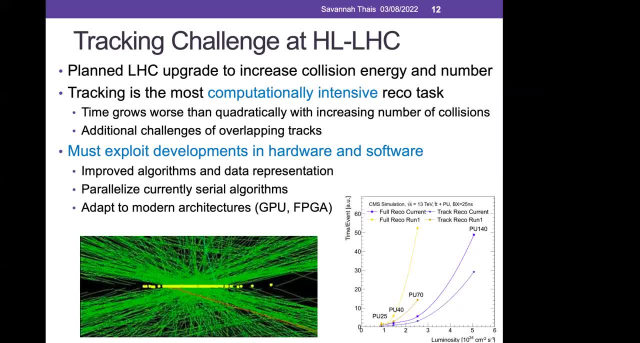 steps. that has to be done, so we really need it to be very accurate so that we're not introducing uncertainty that then gets propagated through the rest of the data processing steps. So it's a very important task, but it's also the most computationally intensive. 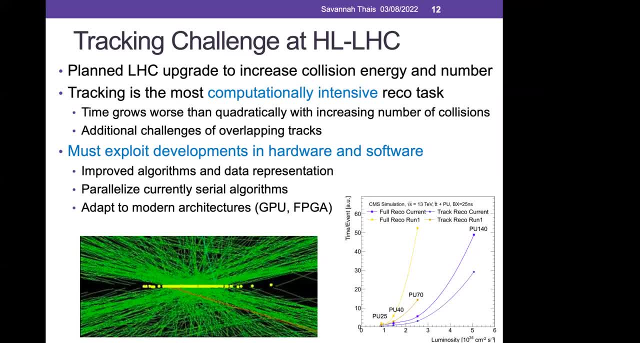 research reconstruction task. that happens with this data And this is a big problem because there's a big planned upgrade for the Large Hadron Collider, where we're going to be producing even more proton-proton collisions at the same time, So the scale of our data is going to really 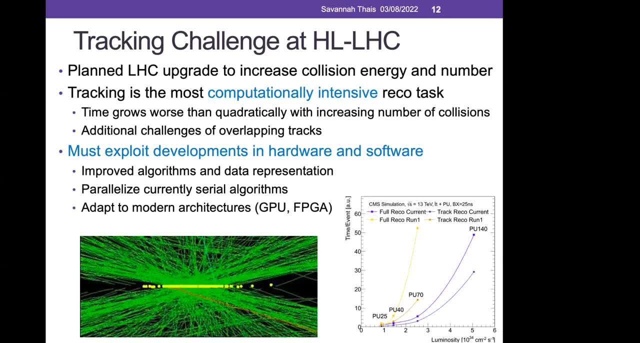 increase And unfortunately, with the current way that this tracking is done, it scales worse than quadratically, with increasing number of particles that you're trying to reconstruct. So as we move through this upgrade, it's just going to become untenable to use the current algorithms. We're not going to have the computing resources to meet. 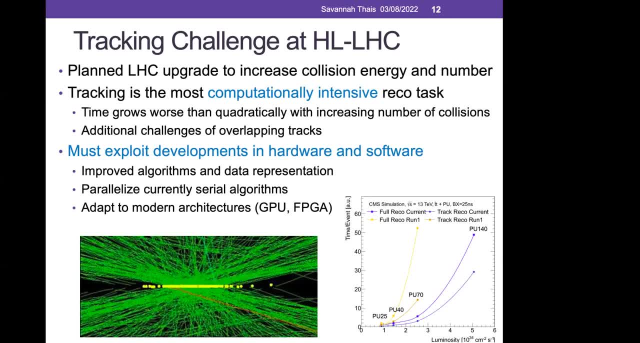 those needs. So we really need to innovate here and try to come up with new types of algorithms, new types of data representations, also ways to accelerate those algorithms. maybe add parallelization, adapt to modern architectures like GPUs or FPGAs and different kinds of things like that. So that kind of motivates why we're. 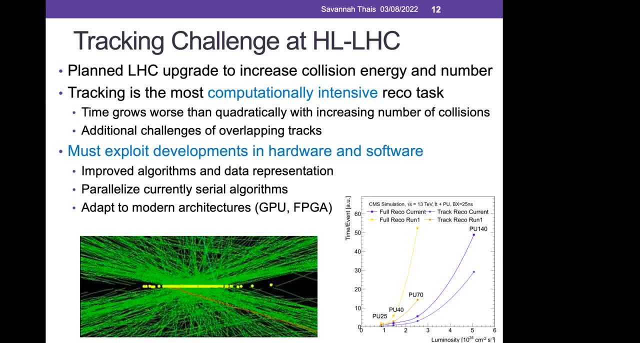 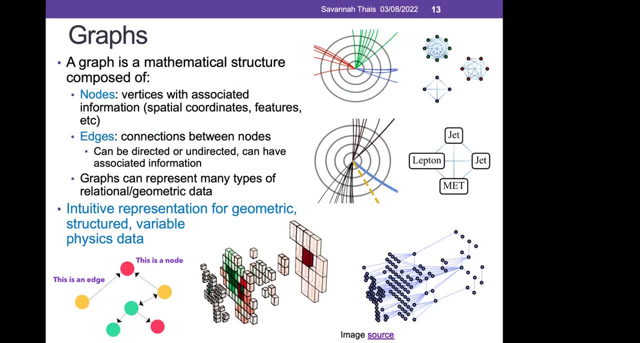 starting looking at graph neural networks for this problem. So graphs, as you might be aware, are a mathematical structure composed of nodes and edges, both of which can have associated information, which could be spatial information or any kind of other features. So graphs can 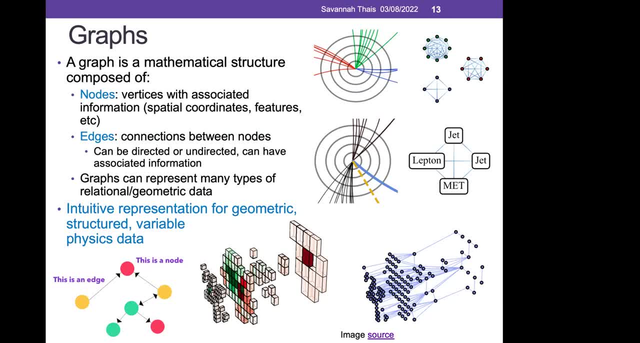 really be used to represent many, many different types of relational or general data. They're used a lot in the physical sciences, beyond just particle physics, also for things like representing protein structures or things like that. but they can also be used for relational data like different types of knowledge, dependencies, social networks. 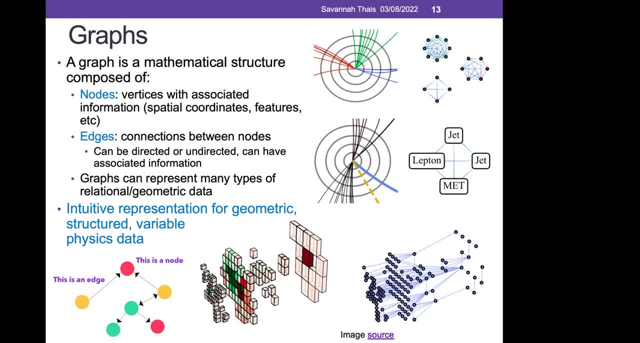 all different kinds of relational structures And they're a really intuitive representation for particle physics data in particular because, like I mentioned, we have variable size data, So it's hard to work with traditional grid-based structures, even sequence-based structures, Like for recurrent neural networks, there's no physical ordering to the data, So 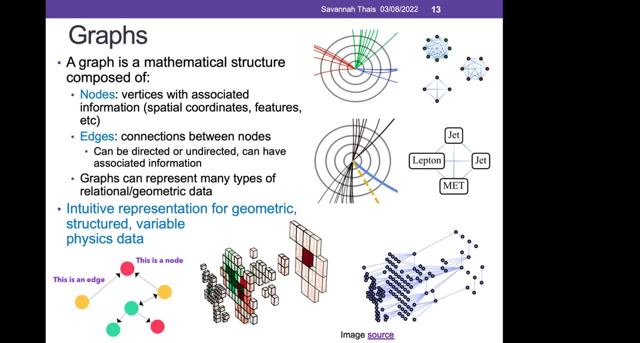 when that has been studied in the past. you have to enforce some kind of arbitrary sequence on the data. So graphs are actually a really intuitive, really appropriate representation scheme for this type of data, And so I think that's really important to look at. And then 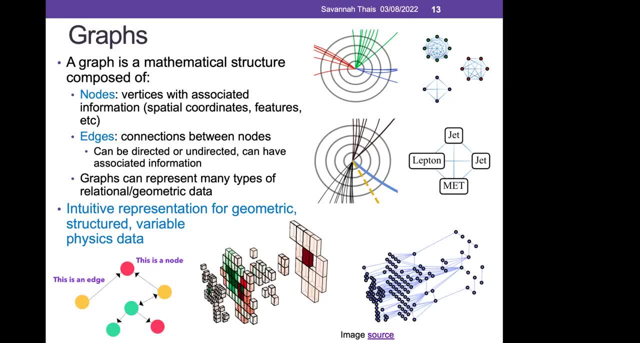 yeah, because of the fixed size and ordering or non-ordering, but also because we know there is geometric component and structure to this data. we know that particles move outwards from the collision point, So there is an inherent geometric structure there, And so I've shown some different. 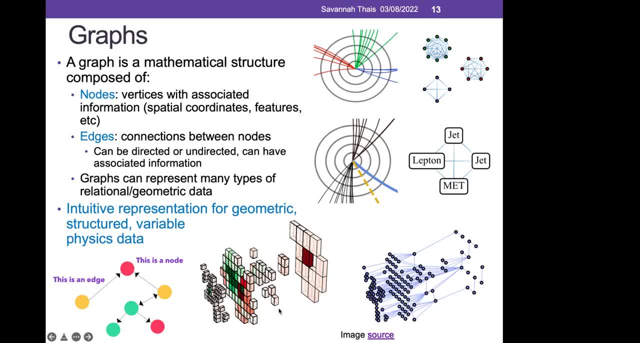 examples here of ways that different types of particle physics data can easily be translated into to graphs. So we have, for instance, energy deposit clusters in what we call a calorimeter, a certain type of detector component We can also represent once we have. 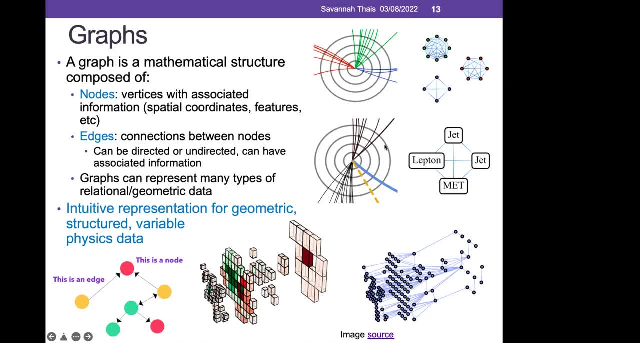 done some of the initial reconstruction stages. we can represent different particle types as nodes in a graph and start to learn. use that to learn about the full physics process that occurred in the collision. We can also use it for grouping different decay products together. 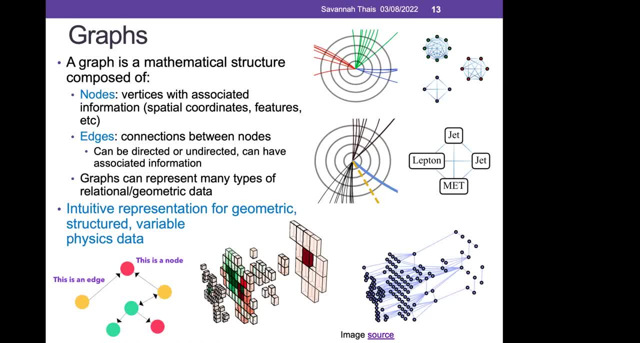 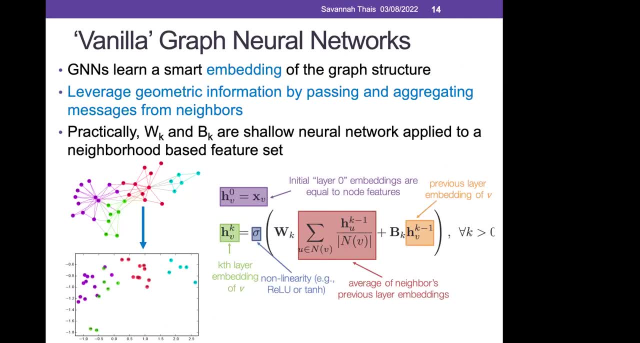 So really a lot of the different kinds of problems that we need to solve in particle physics, it makes sense to use these graph representations. So once you have a graph representation of your data, you need some kind of algorithm that can operate on that structure and really exploit and make. 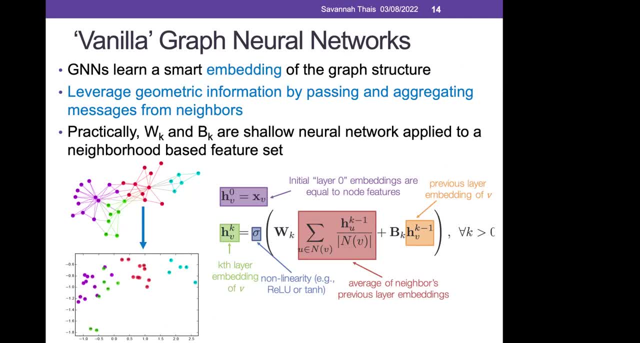 use of these nice features that I just described, And so the most vanilla version of graph neural networks or message passing networks kind of work like this: They try to learn some kind of smart embedding of the graph structure where you can then do some downstream tasks like node classification graph. 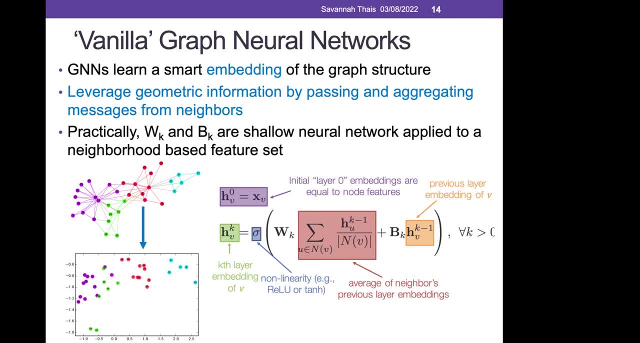 level, classification, graph segmentation, different things like that- And they work by leveraging geometric information from the graph. OK, So in this case we have some sort of graph that we can do with this kind of works like this, So the kind of most vanilla version of graph, neural networks or 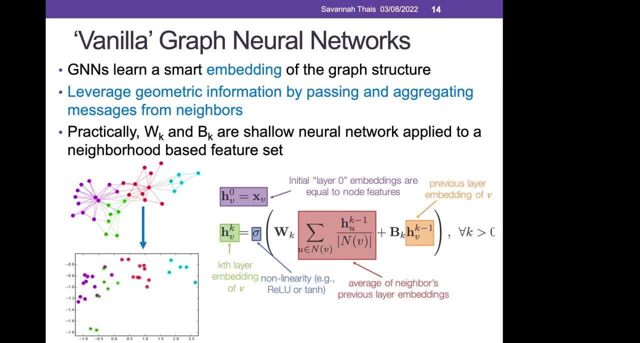 by passing and aggregating messages from a graph's neighborhood. So I know some of you might have seen it. I've seen GNNs be familiar with this, but I'll just quickly explain them anyways. So in a node-based message passing GNN, what happens is you have some initial embedding for a particular 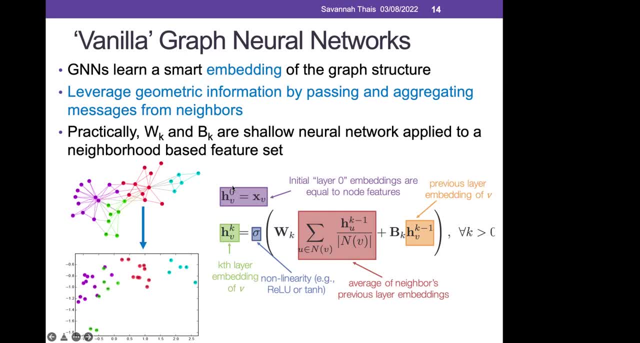 node, which would typically be just the initial features of the graph node, and then to re-embed that node or update its features, you apply a feed-forward neural network to the aggregated information from all of the other nodes that that node is connected to. So you collect the previous. 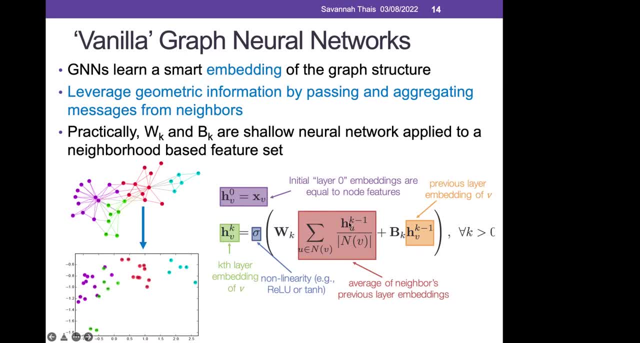 embeddings of the node, of all of its neighbor nodes. you do some kind of aggregation here. it's averaging, but you can do different types of aggregation and then you can apply some transformation to that. Here we're also including a transformation of the node. we're 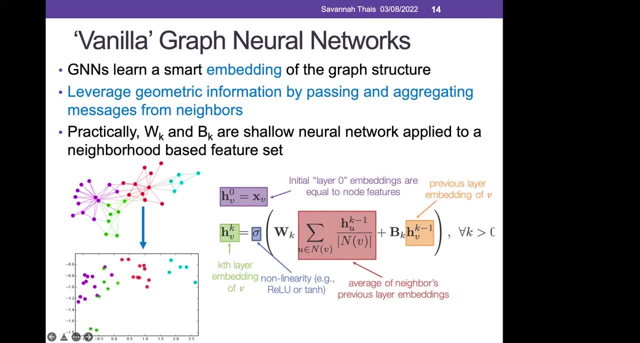 updating its previous embedding and then you apply some non-linearity to that And there's lots of modifications that people have looked at on this kind of basic structure You can use- you know- different types of aggregation, you can do different types of aggregation and then you can. 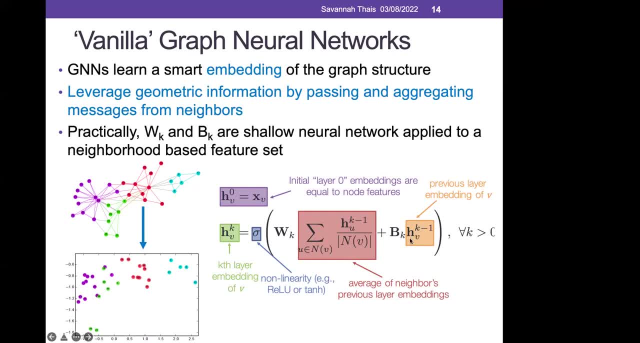 add different kinds of information. you can drop this previous node embedding or add other types of information. use different types of aggregations. you can add, you know, different neighborhood combinations, things like that. there's lots of different modifications that can be made. 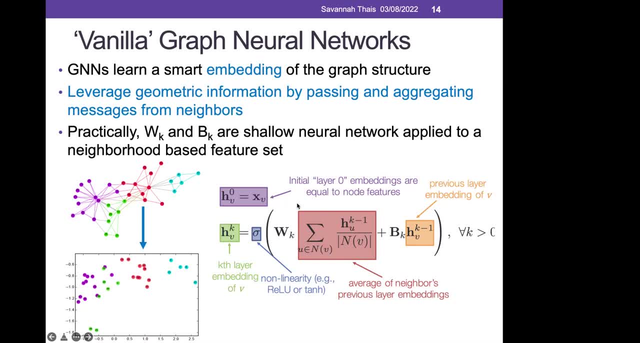 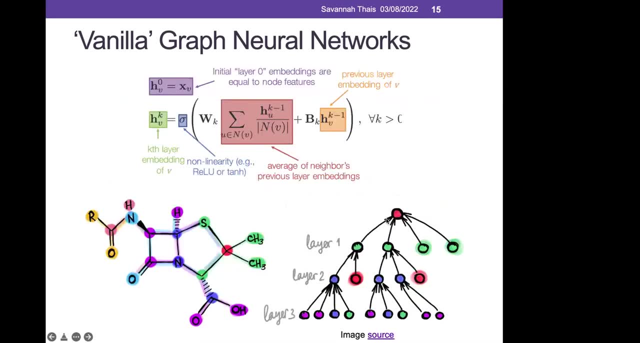 But this is kind of the core message passing structure that really makes the foundation of a lot of other GNN architectures, And so what's really interesting about GNN is that you can do a lot of different things with it. So what's really powerful about these is that, by combining, 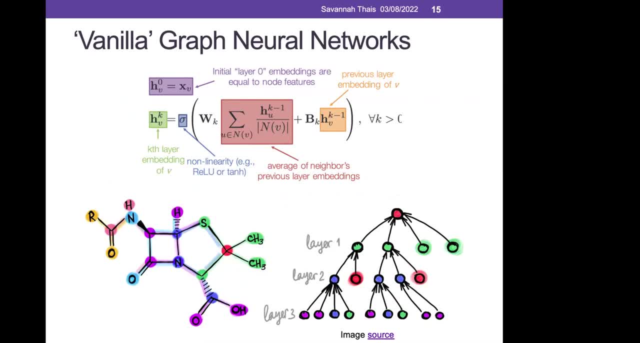 these, embedding multiple of these graph layers, we can start to collect information from farther and farther away on the graph. So that's kind of what's shown down here. So if we're looking at updating this red node with the first graph convolution layer, we get information from its. 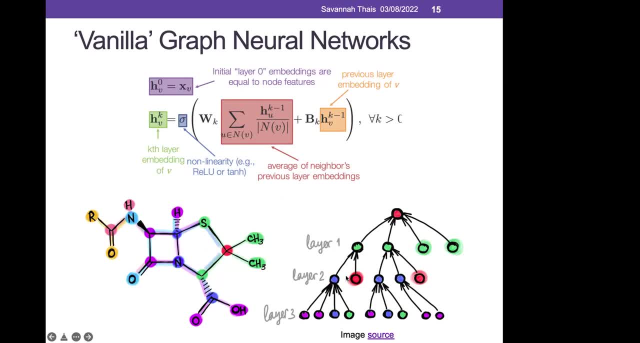 immediate neighbors, these green nodes. As we add another graph, convolution layer, we get information from all the green nodes neighbors, which include these blue nodes, but also previous information about the node that we're actually trying to learn about, And then so on. for the third layer, you get information from the blue. 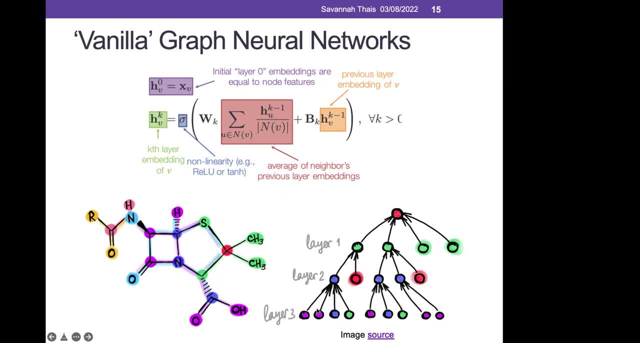 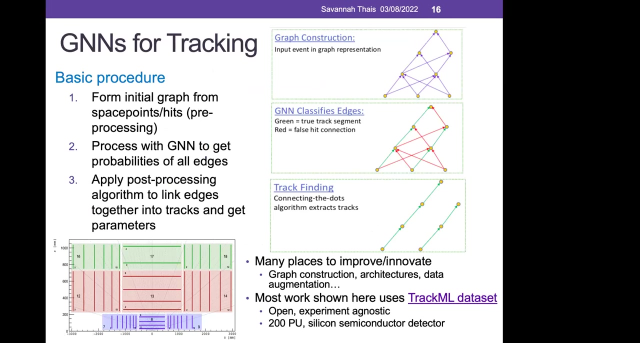 nodes, neighbors, which include the purple ones, but also again then the previous embedding of the green, the green nodes. You can see how you start to progressively capture a lot of relational information from the graph. So how do we use this for that tracking problem I was talking about? So we've looked at a lot of 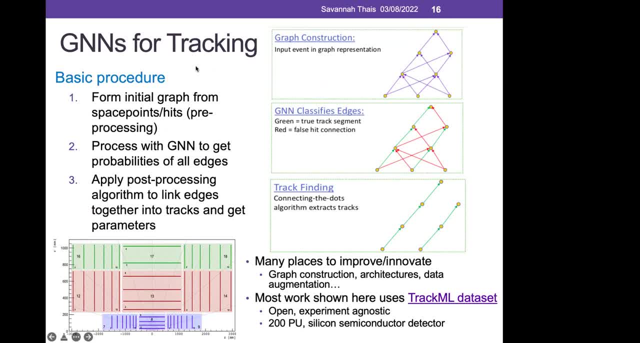 different methods that I'll talk about in a few minutes. But the kind of most basic structure we've applied is that you form an initial graph and I'll talk about different ways we can do that graph formation from the initial graph and I'll talk about different ways we can do that graph formation. 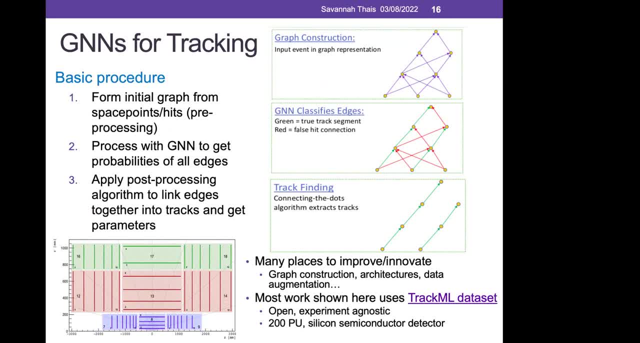 from the initial graph- and I'll talk about different ways we can do that graph formation from a hit cloud or from a point cloud of hits in the tracker. Then you process that graph through some kind of GNN to get probabilities on the edges. So we want to try to figure out if the edges in 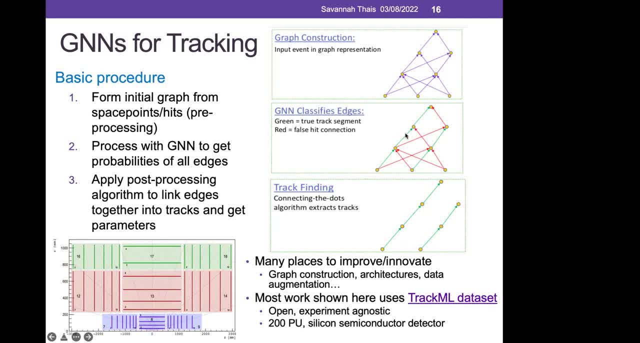 the graph represent real particle trajectory components or, if they're just noise edges, false edges. So we use the GNN to get edge weights or edge probabilities And then we apply some kind of post-processing algorithm to link those classified edges together into final track. 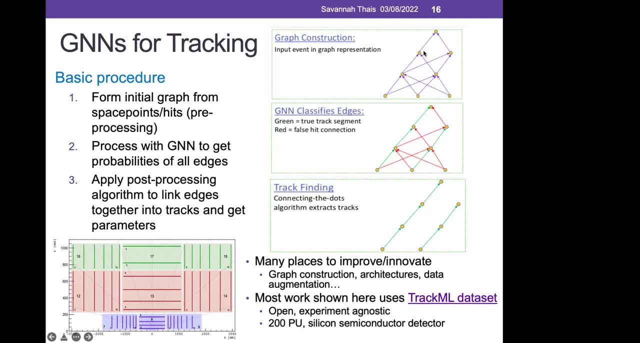 candidates. So you can kind of see how that looks like here in a very small scale example. So we have some initial graph. We want to learn about these two. We want to learn that these two variables are real particles. So we want to learn that these two variables are real particles. 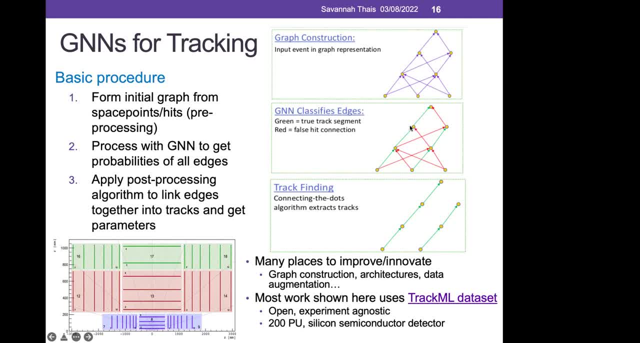 So we want to learn that these two variables are real particles, So we want to learn that these two green lines are the true particle trajectories. So our GNN would hopefully learn to downweight the red segments and upweight the green segments, And then these are already distinct clusters in. 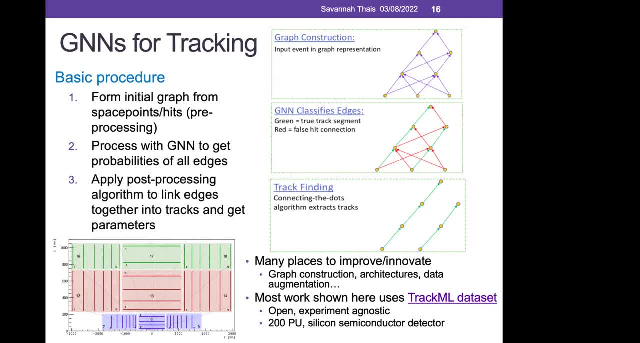 this example, but in more complex data situations you would have to do some kind of clustering as a final step to identify the final track candidates. So this is the very basic architecture that we've started with, but there's a lot of places to really build on that. 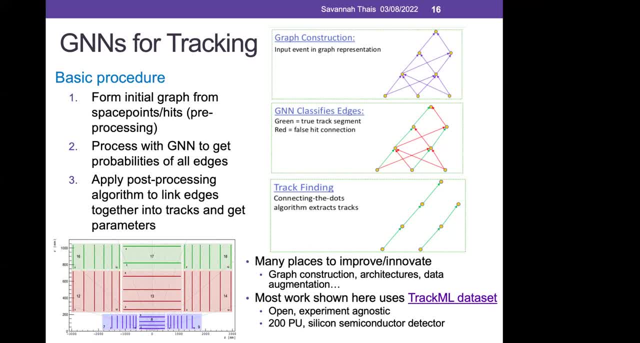 So we're going to talk about some of the ways that we've been doing that And then just to note, the work shown here uses this track ML data set, which is an open source data set available to anyone, So you could go run, play around with it right now if you want to. It's based on a detector. 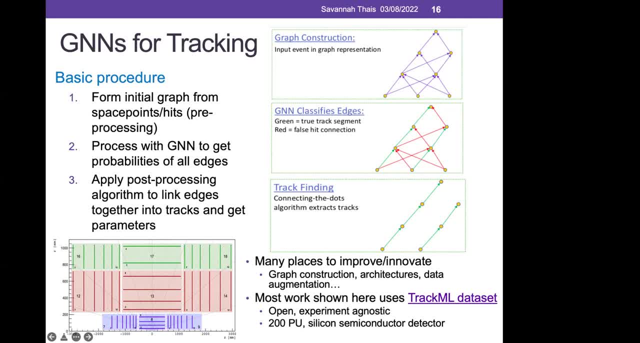 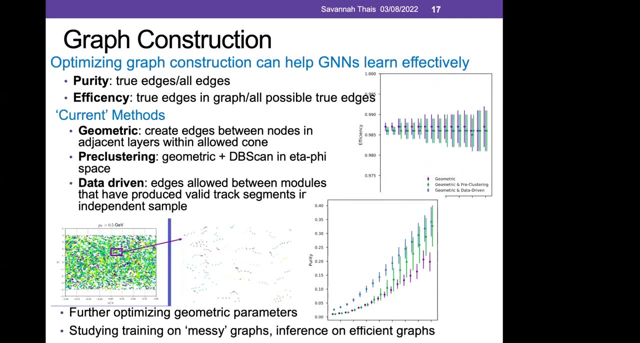 from the Large Hadron Collider, So it has the same geometry but it's open source data, So it's really easy to collaborate with different machine learning colleagues as well as kind of traditional physics researchers. So the first step in that pipeline, like I mentioned, is graph. 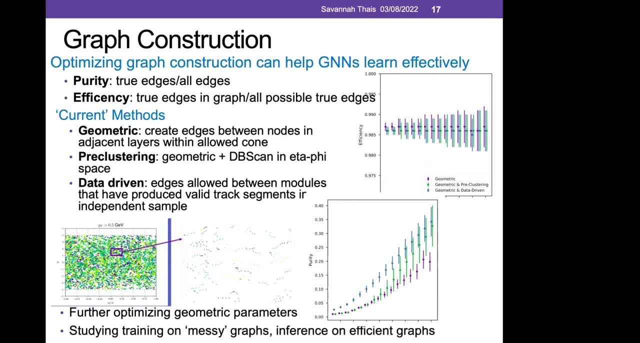 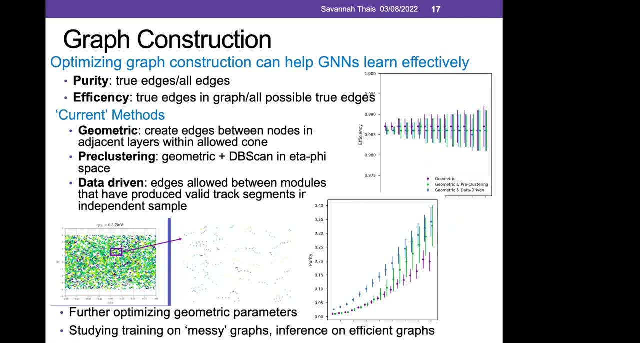 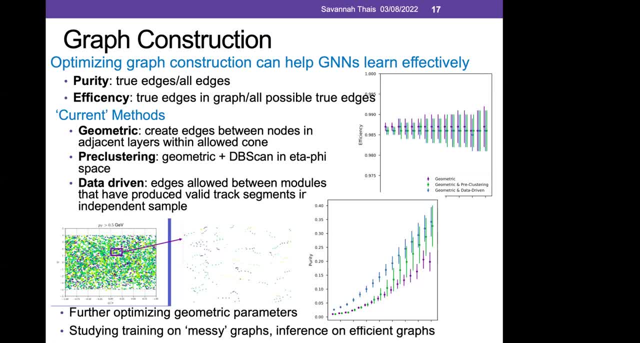 constraint. So we only allow, we allow all connections between adjacent layers of the tracker, but within some physics driven cone space. So we don't, you know, allow connections between one part of the structure and the other part of the structure, So we don't allow connections. 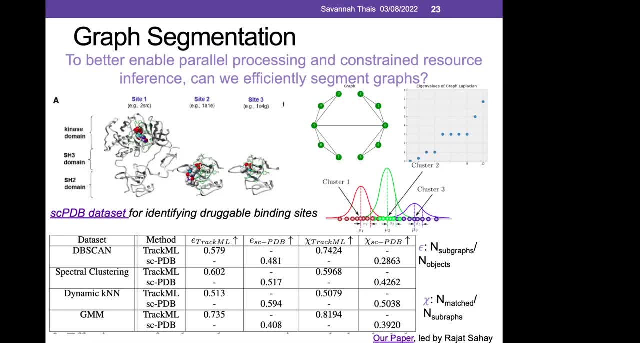 between one part of the structure and the other part of the structure. So we don't allow connections between one part of the structure and the other part of the structure. So we don't allow connections. it connects the k nearest points to a particular node, but with the dynamic component. 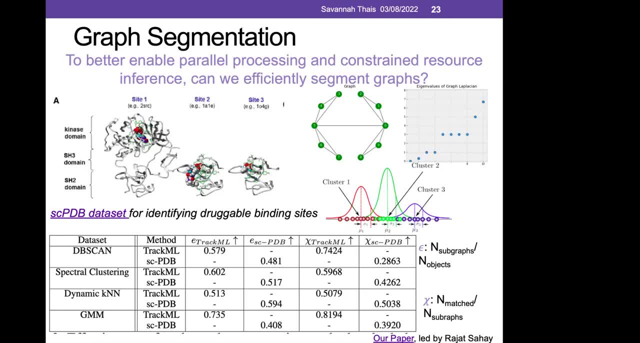 you can vary the number of clusters that you're creating. and then we also looked at Gaussian mixture models, which have the assumption that your data is generated by some kind of Gaussian process and it tries to figure out like the optimal generating Gaussians for your data set. and again, 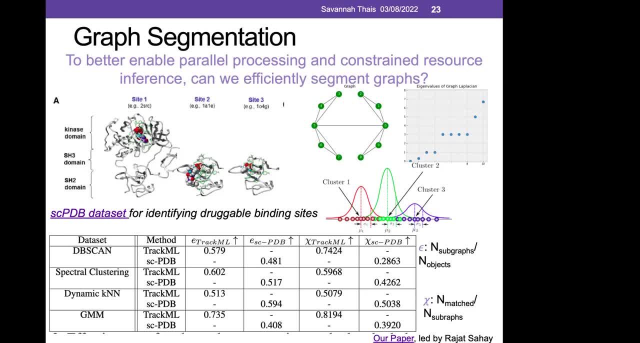 that allows a variable number of clusters to exist. So we looked at these different clustering algorithms for both the track graphs and the protein graphs, and we looked at two measurements to try to describe how well these are doing at effective segmentation. So we look at efficiency, which is the number of subgraphs you get out of your clustering, compared to the number 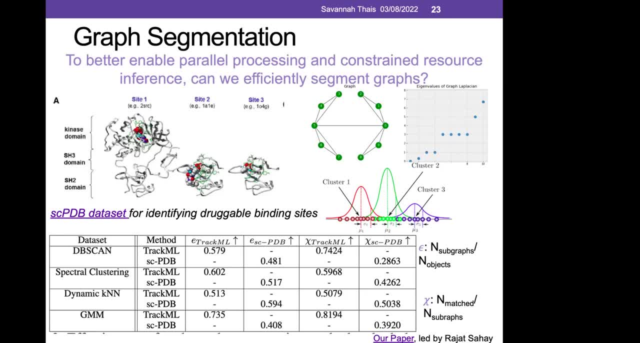 of objects, so either tracks or binding sites. And then we also looked at this chi value, which is the number of matched subgraphs to truth value. so it would be the number of track candidates that actually sorry, the number of subgraphs that are individual particle tracks, or the number of subgraphs that are distinct binding sites. 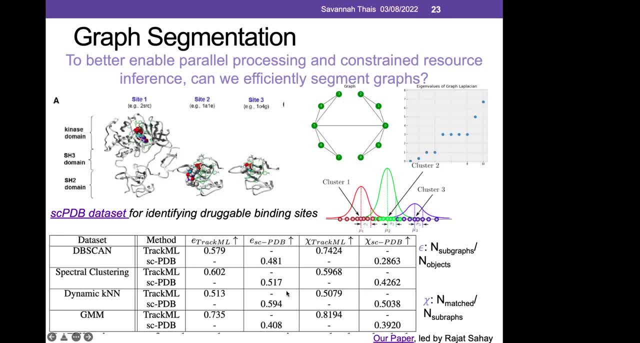 over the total number of subgraphs And we found that Gaussian mixture models do really a sufficient job at segmenting the track data sets. We get almost 75% like distinct subgraphs compared to the number of tracks that should exist, and 80% of those are individual particle trajectories. 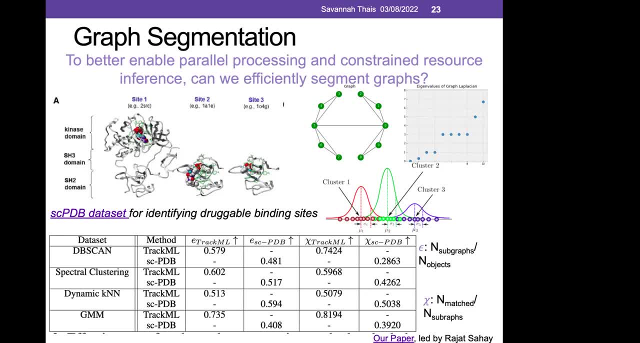 So we're getting like around. that would be like 60% of the integer trajectories we're trying to find. We already distinguish them before even doing any kind of GNN processing. For the protein data set. the results were not quite as good. We saw that like dynamic KNN. 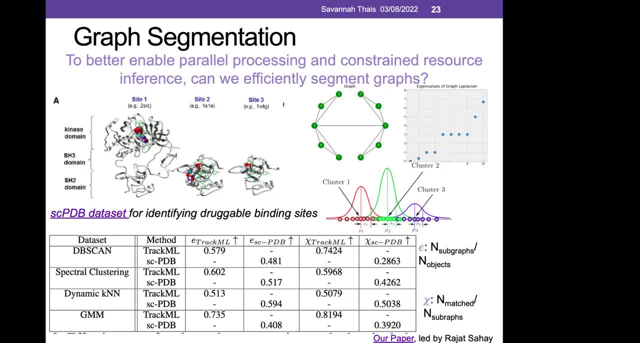 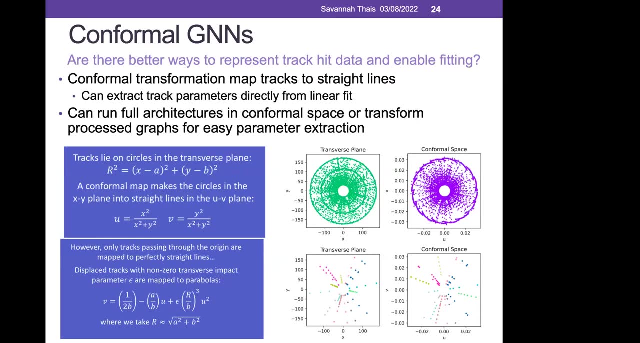 does the best job at graph segmentation, but they're only about 50% accurate, so you would definitely need some more processing for that, but you can still start to parallelize the inference Then. this is not necessarily its own study, but just something that I'll talk about. 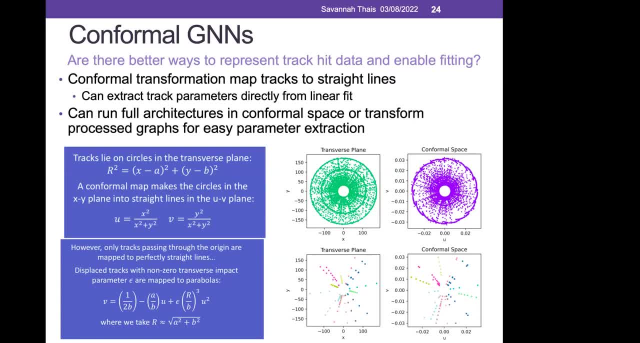 for some of our other studies We were thinking about if there are better ways to represent the track hit data and enable track fitting. So there's this alternate space called conformal space that is really useful for representing some particle data in that basically maps those helical tracks to straight lines or parabolas, depending on. 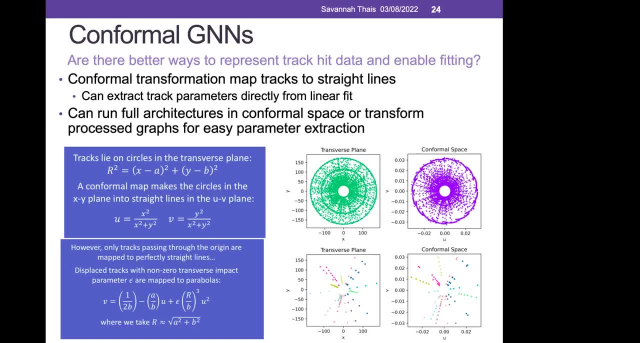 if the track was created at the interaction point or somewhere later in the detector, This transformation can be really useful. We're looking at both running full GNN architectures in this space instead of traditional euclidean space, to try to see if it's easier for the GNN. 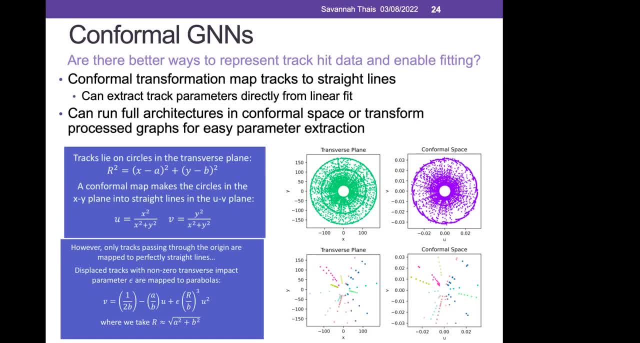 ends to learn in that space where tracks are straight lines Or we're also looking at after we've done the GNN inference and we've built these track candidates, if we can use this conformal transformation to do easy track fitting So you could just have your track candidate. 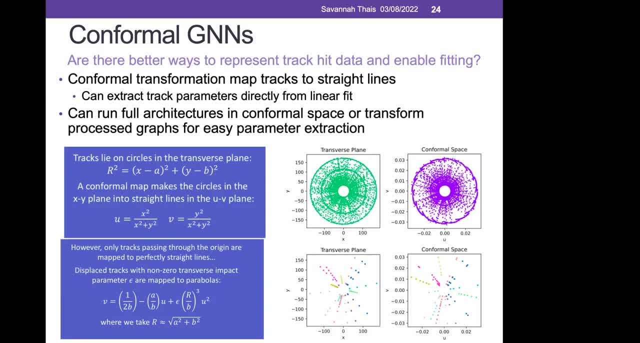 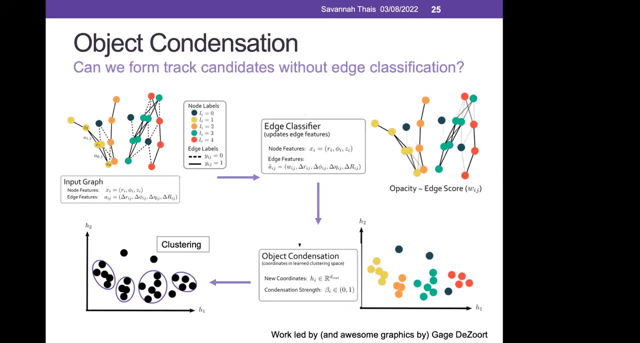 from the dbscan, clustering or whatever. You can just fit it to a straight line and extract track parameters. We're looking at both of those ideas. So another approach that we've started looking at for this GNN-based tracking is called object condensation, where 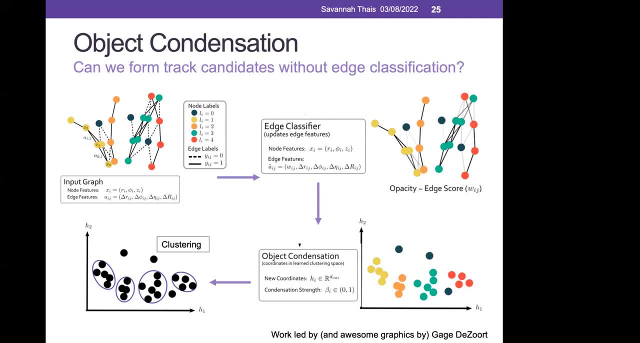 we're trying to look at, can we form those track candidate clusters without doing full edge classification, so without actually removing edges from the graph, but just getting edge weights and then using those edge weights in a smart way. So the pipeline kind of looks like this. 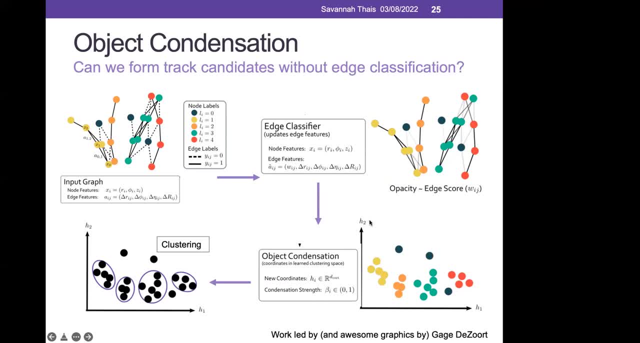 We add this additional object condensation step to our original GNN pipeline. So you have your input graph, then the edge classifier that predicts some edge weights. Then you use those edge weights to help move data points that belong to the same track. So you can see here that we have the same track closer together. 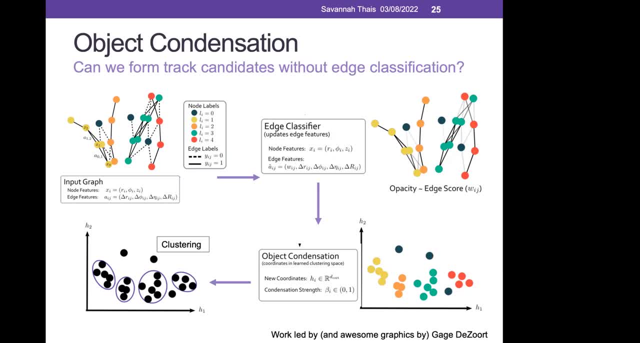 in this new learned space and to repel ones that don't belong to the same track away from each other. And then you still have to do this final clustering step. But perhaps your clustering will be more efficient once you've done this. object: condensation. 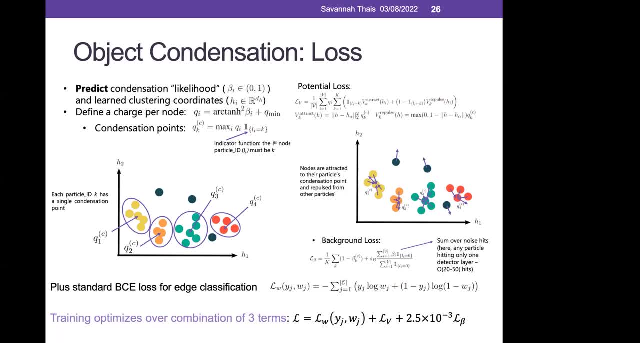 So to do this object condensation approach, we have to modify our loss function by adding some additional terms. So we have our standard BCE loss for the edge classification, like we use in our normal pipeline, but then we add some additional terms that we're trying to predict. 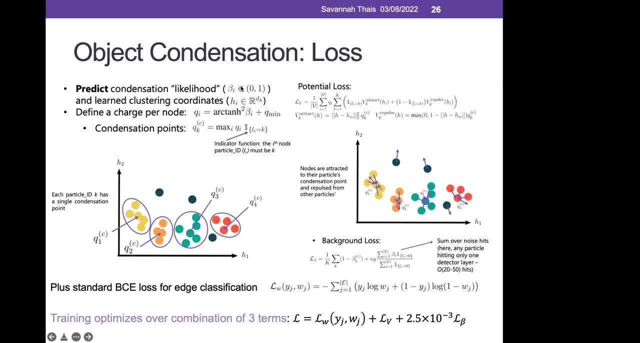 So we're trying to predict the condensation likelihood of each node and a learned clustering coordinate. So we're learning a new embedding space for the graph and then we're predicting a likelihood that it belongs to a certain condensed cluster. So at the truth level we define these condensation points. 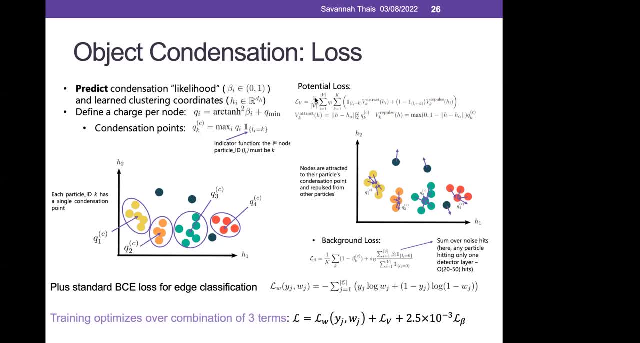 that should exist for each track And during training we try to learn good GNN convolutions that move points towards their truth, condensation point, And so we have a potential loss that combines an attractive term that tries to pull related points together and a repulsive term that tries to push. 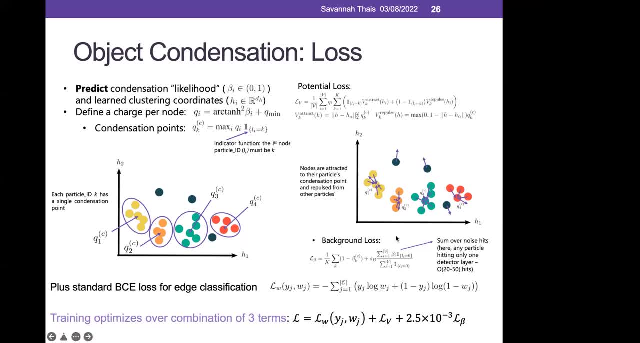 unrelated points apart. And then we also have a background loss term that seeks to distinguish any nodes that don't belong to any actual tracks and to try to separate them from everything else. So our full training optimizes over the combination of these three terms, where the background loss is really. 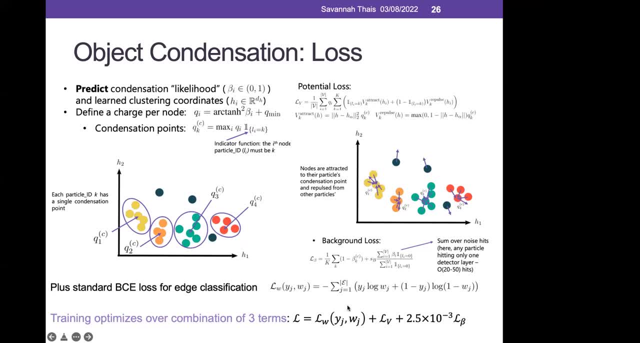 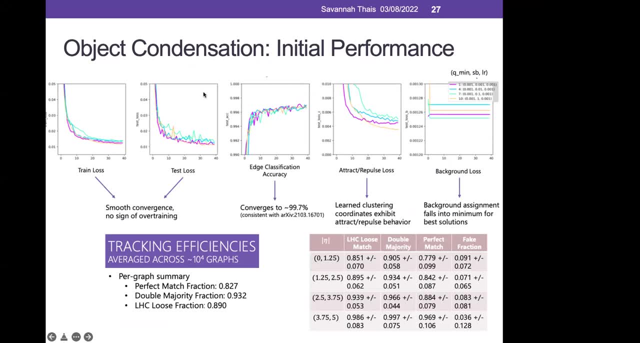 downweighted Compared to the other two because it's not quite as important, at least in this particular data set, And we've seen some really promising results from this. already We get comparable edge classification efficiency to our previous architecture and good convergence of the attractive and repulsive loss. 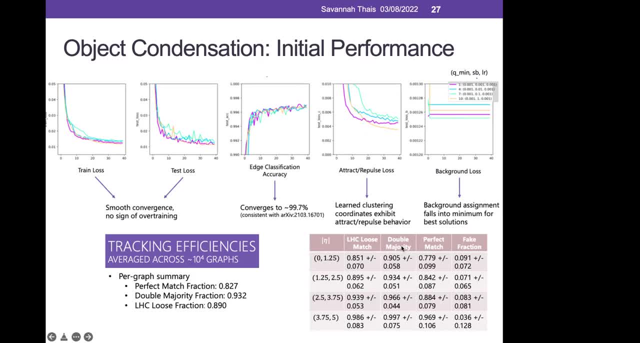 as well as the background loss, And we see some really promising results from this already And we see, when we do the full tracking efficiency calculation, pretty similar performance to just the standard pipeline, but we actually get lower fake rates, which means we're identifying fewer false tracks, which 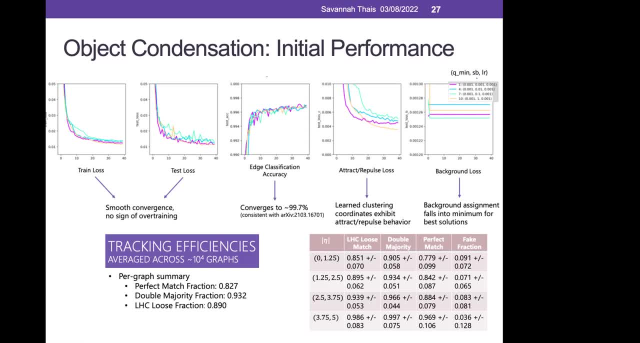 is another really important consideration for doing tracking in these kind of detectors, And this hasn't really been optimized at all, So we're going to have to do a little bit more work on this, So it's a really promising direction that could potentially even surpass 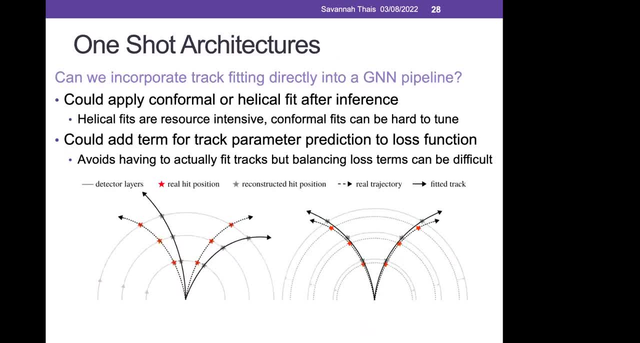 the kind of interaction network approach we've been looking at. Then another idea we're looking at is what we are calling one-shot architectures, where we try to incorporate track fitting directly into the pipeline. So right now, with both the object condensation and the interaction network architectures, 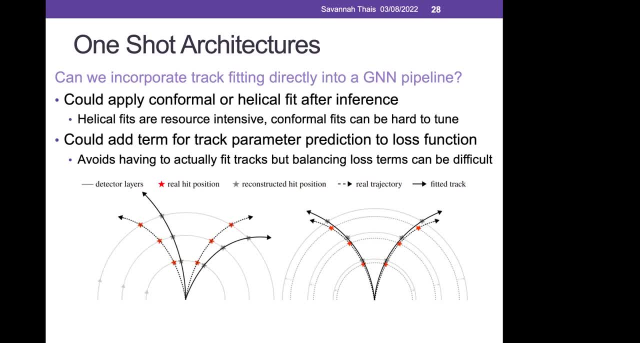 we only get out track candidates And the final step in doing tracking is getting things like the momentum and the vertex of the track. So we're interested in trying to do this directly in the GNN And so you can apply, like I said, a conformal fit. 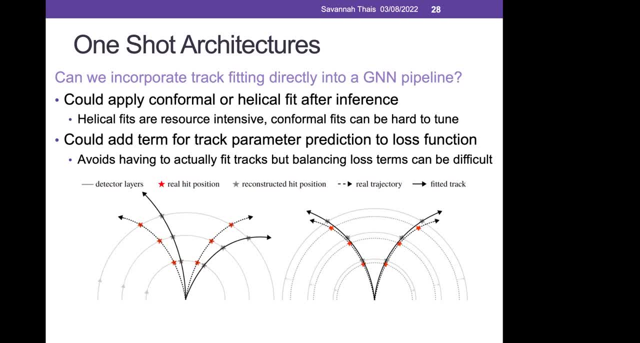 after you do the track after the GNN inference. But what we're really interested in is adding a term to the loss function that could actually be applied to the loss function, And so we're going to do that. That could do track parameter prediction directly. 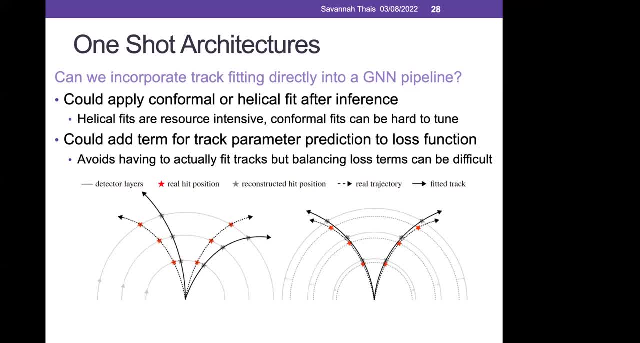 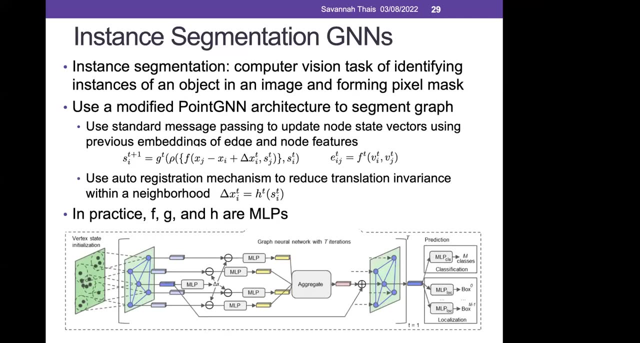 So we've started looking at that. Unfortunately, no real results yet, because it's quite difficult to balance so many loss terms we're finding. But that's the direction we're looking to move in, And then I'm going to skip over, I think, these few slides. 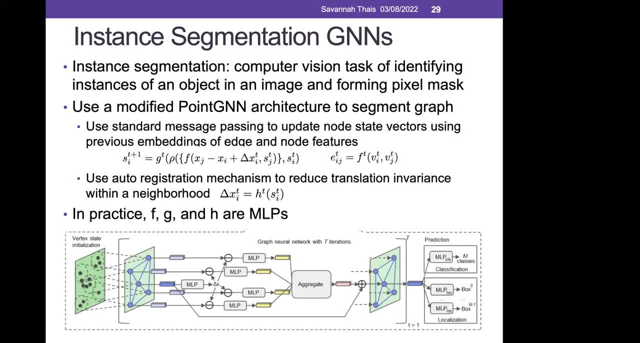 But this is basically talking about an architecture that we've been looking at. So we're looking at to try to do an attempt at this one-shot tracking approach where we incorporate the track parameter predictions And it's based on a instant segmentation bounding box architecture where, instead of doing edge classification, 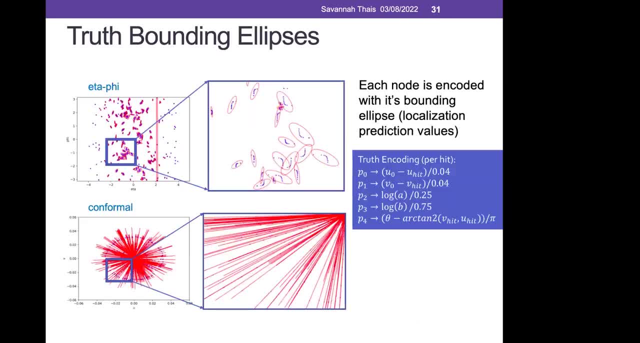 we try to identify bounding ellipses that separate in particular individual tracks from each other. So this is what's done in a lot of image recognition in standard machine learning, typically with boxes. Here we've done ellipses because it fits better with the shape that these particle tracks come in. 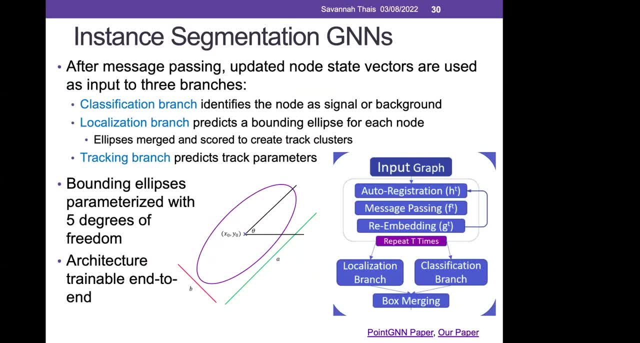 So basically what we do is we define a bounding ellipse for each track And we encode that with the individual node location. So for each node in the graph we're trying to predict the ellipse that it should belong to. So our full network structure has three different branches. 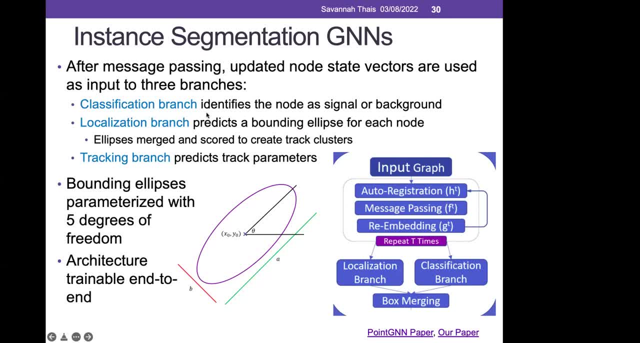 We have a classification branch that's doing that background classification, like I mentioned in the object condensation architecture. Then we have the localization branch that predicts the bounding ellipse for each node. Then those are merged to create our final ellipses. that should separate each track. 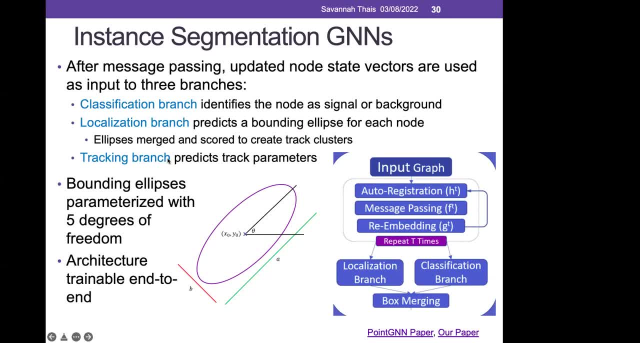 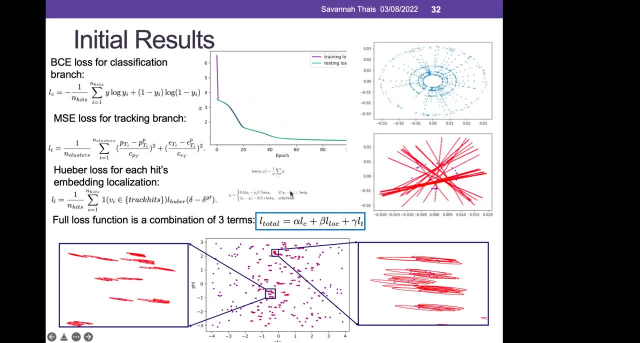 And then we have a tracking branch that predicts the track parameters, And so the final loss function is a combination of each of those three goals, And you can see some very preliminary results here. We looked at both conformal space, which is what these two 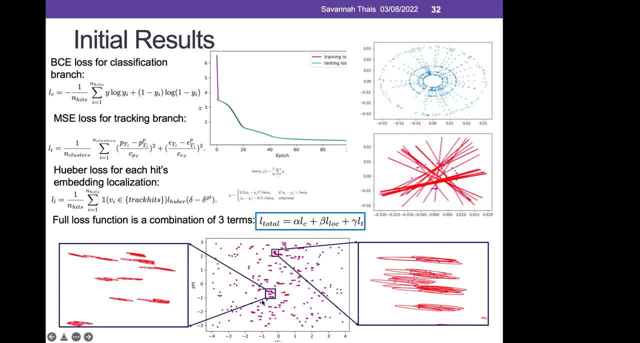 plots are showing, and then just Euclidean space, And it works fairly well. in Euclidean space We definitely get some overlap between nearby tracks, So we're still trying to fine-tune our merging. Unfortunately it doesn't seem to work in conformal space. 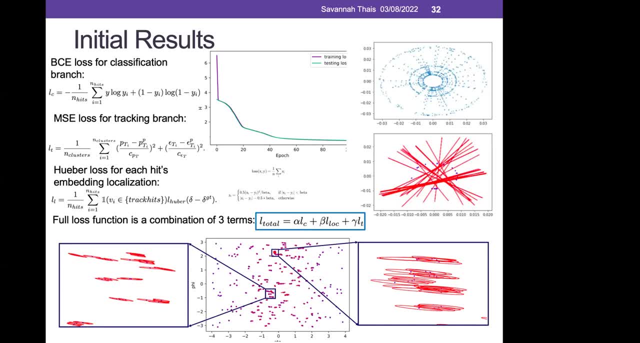 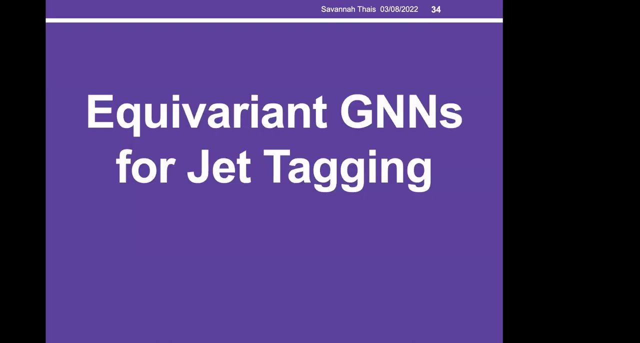 because the ellipses are so stretched out in that space It seems to be hard for the GNN to really learn the parameters efficiently. But we're still doing ongoing work on this project And I linked to our first paper about it And then, quickly, I want to talk about this last paper. 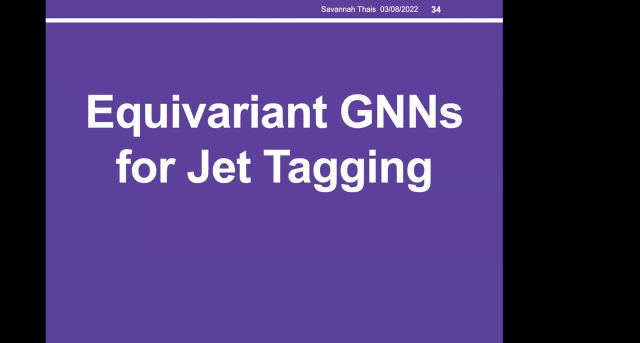 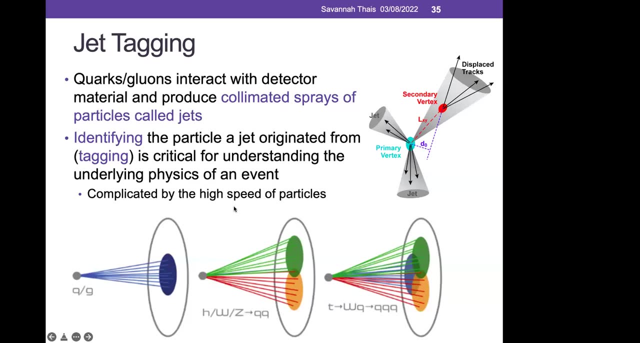 that we recently put out, which is on a different topic, but still using GNNs for reconstruction. Sorry to interrupt you, Savannah. Yeah, it's just because we have 10 minutes. We have 10 minutes left on the presentation. 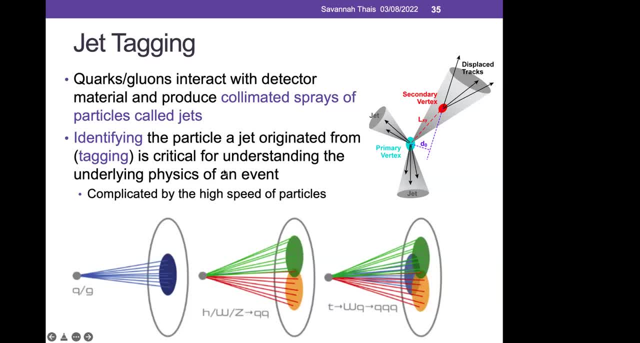 If we can leave some 10 minutes for people to ask questions. OK, Yeah, I'll just go through this really quickly, if that's OK. So here we're looking at, instead of doing trajectory finding, looking at grouping, decay products of a particle. 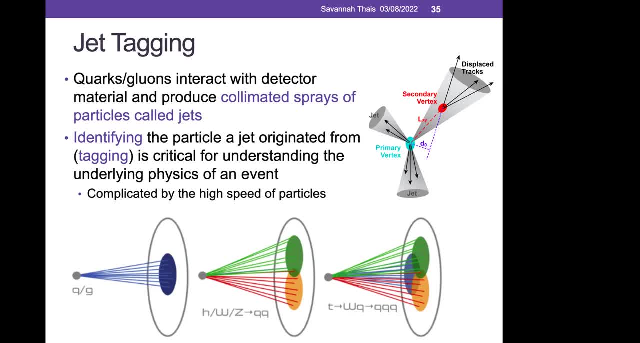 together And then identifying the way that we're going to do this, And then we're going to look at how we're going to do this, And then we're going to look at how we're going to do this. So here's an example. 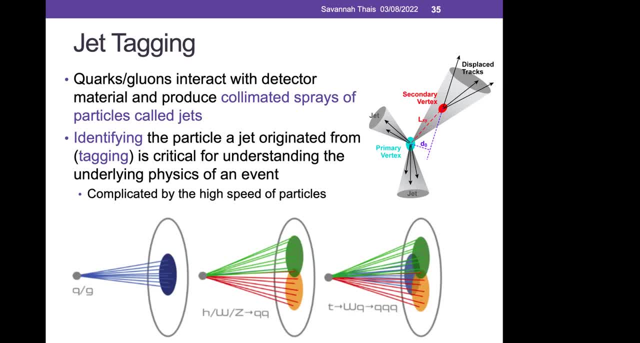 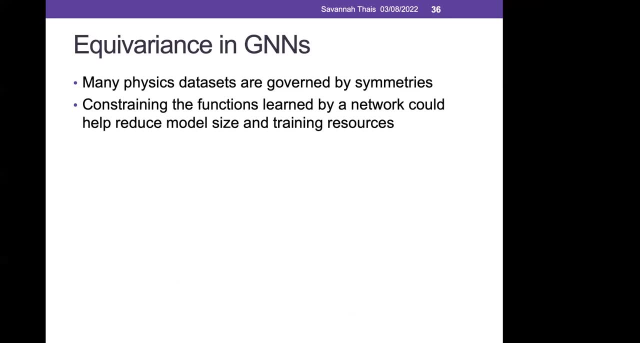 So this is a physical particle that that decay spray came from And sorry, I had a lot of computer issues So I didn't really finish this slide. But basically an idea that has been kicked around a lot is that particle physics and a lot of other data sets. 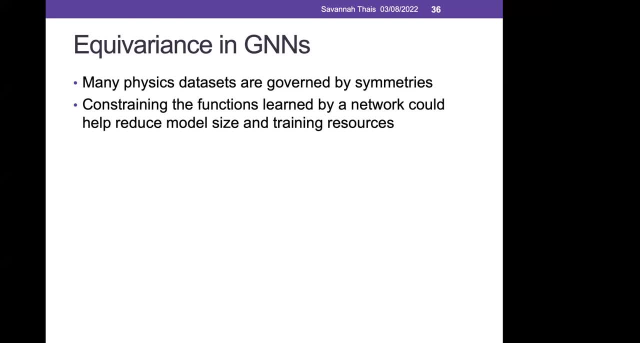 as well, are governed by symmetries that dictate how the particles should interact with each other, how they should decay, And so there's an idea that constraining The functions learned by a network can help reduce the model size. you need fewer parameters to learn the appropriate classification function, and you can also reduce the training resources needed to develop the full pipeline. 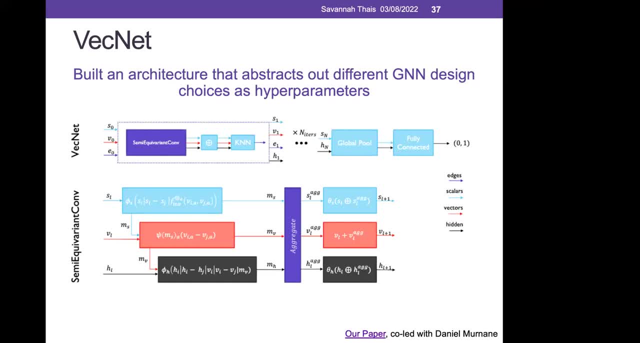 So in the paper I linked to here, we introduced this new architecture, VecNet, that abstracts out both the idea of equivariance but also other components of GNN, architectures for physics tasks like your graph construction method, your aggregation method, these different kinds of things. 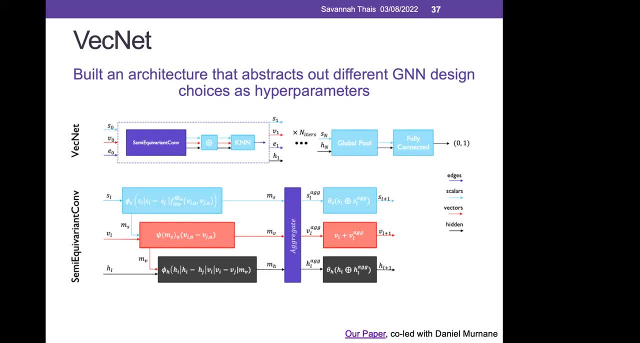 And so we abstract out all of those as hyperparameters And we allow for equivariant information to flow. We allow for equivariant information to flow through the scalar and vector channels that propagate equivariant scalars and equivariant vectors, and then we have a separate hidden channel that just allows any type of information to flow through the network. 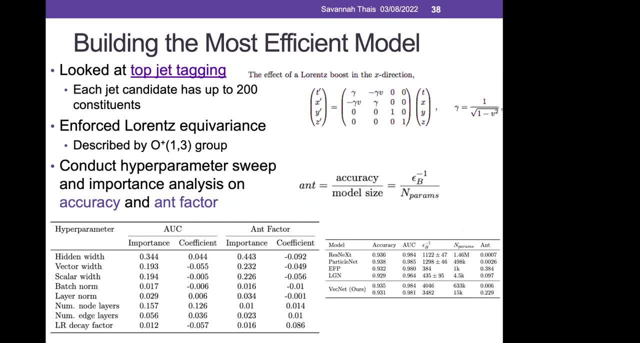 And what we're trying to figure out is if equivariance, what impact equivariance actually has on a model, if it does allow you to build more efficient models or not. So we studied a particular type of jet tagging problem And we looked at Lorentz invariance, which is a type of fueled subtleties. 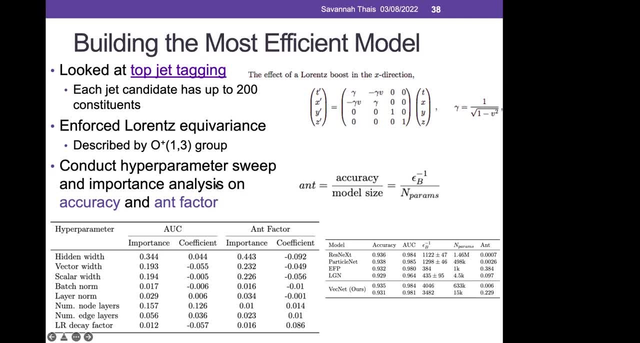 symmetry that all relativistic particles, so very high energy particles, should obey. We looked at the impact of equivariance and these different hyperparameters on both the accuracy of the model but also this amt factor, which compares the accuracy to the size of a model. 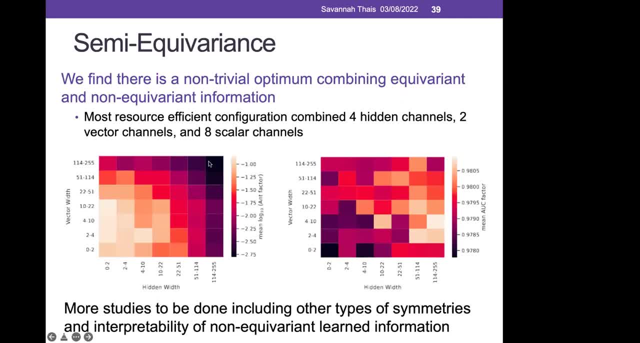 And The kind of interesting result that I want to highlight here is we found there seems to be a really non-trivial optimum that combines some amount of equivariant information with some amount of non-equivariant information And for this particular task, the most efficient configuration we found combined four hidden channels, so four channels of non-equivariant information, with two vector channels and eight scalar channels. 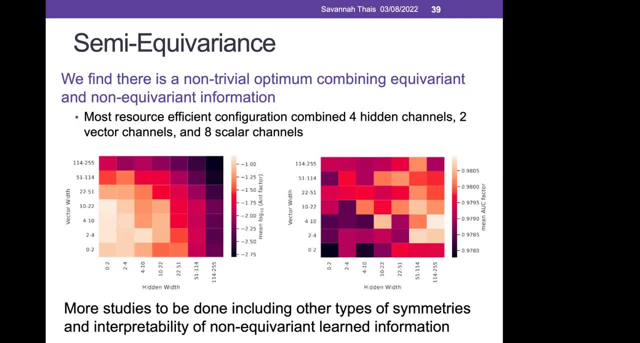 So it seems that allowing some amount of non-equivariant information into your model helps increase the accuracy, but having the bulk of your information be have this enforced symmetry can help constrain the model size. So this is a really interesting direction that we're still pursuing. 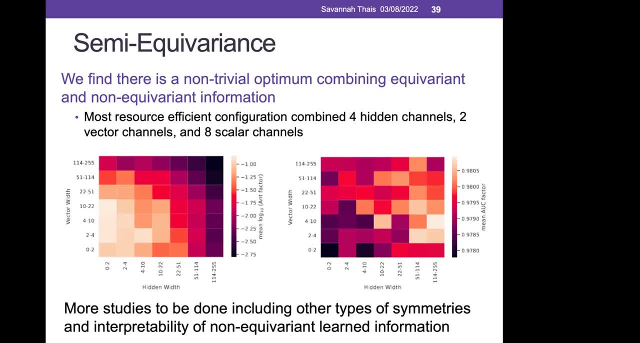 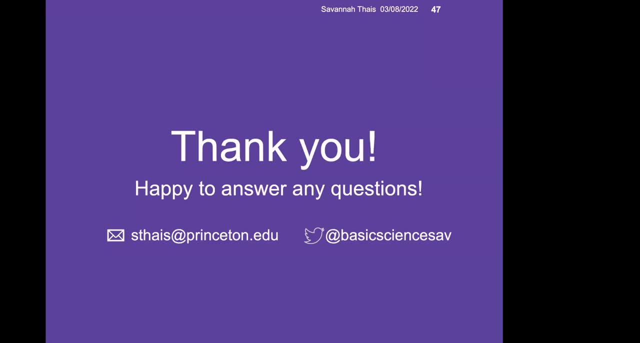 We're looking at different types of symmetry, beyond just the rent symmetry, and then also trying to bring in some interpretability methods to look at what is being learned by these hidden channels. So I will stop there and, yeah, happy to take any questions. Thank you so much. 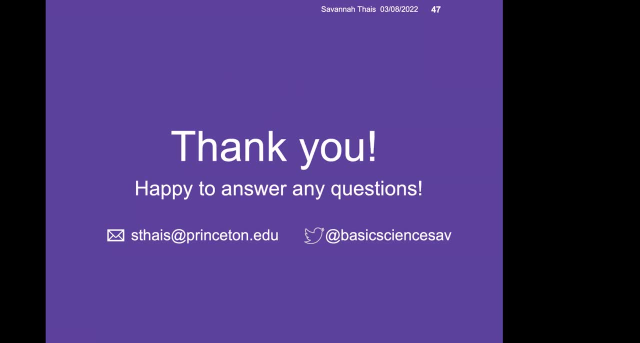 Thank you, Savannah. So I'm going to take some questions from the audience. So raise your hand so you have questions, Otherwise you can type it on the chat. I'm going to take the first two questions. Santiago on slide 17 was asking- this is very specific: what's on the x-axis? 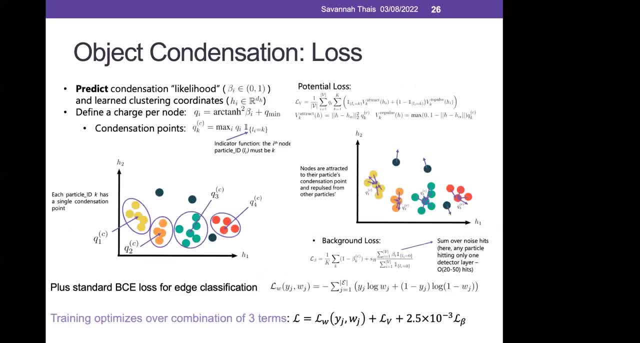 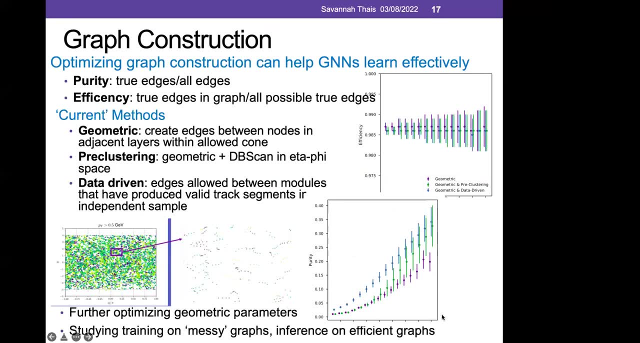 Slide 17.. Let's see. Oh, sorry, So this is momentum of the track. Yeah, thank you. We have another question. I think it was slide 19.. Can we have the slides? if you can share the slides Basically, so he can get the paper link on the slides. 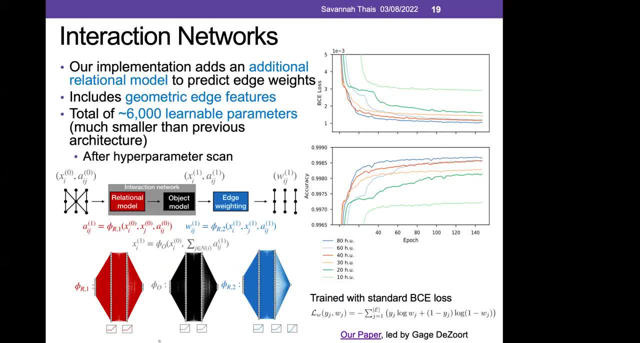 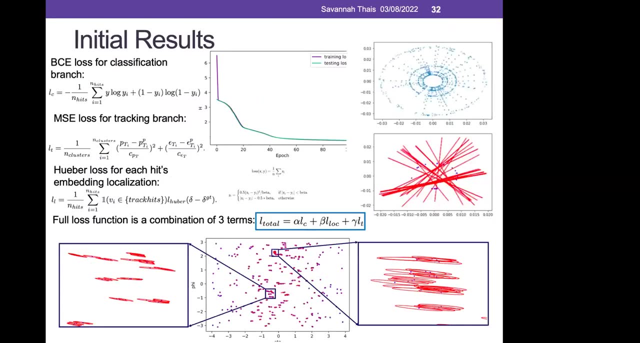 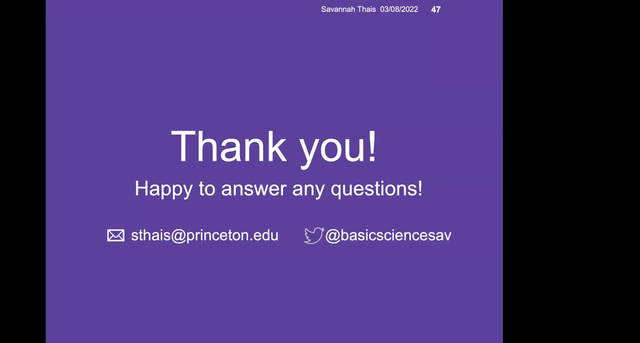 Yeah, Yeah, I'm definitely happy to share the slides. Okay, Thank you. If anyone else has any other questions, please raise your hand and I'll give you the floor. There's a question in the chat. What are the graph neural networks trained on? 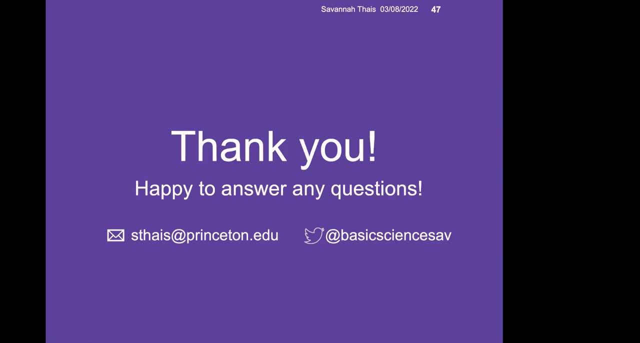 Are they simulated on Monte Carlo data? Yeah, Yeah. So right now all of the data is simulation, because we need the true labels, So we want to know actually what process all this data is originating from, what the track components, track parameters should be, or what the jet labels should be. 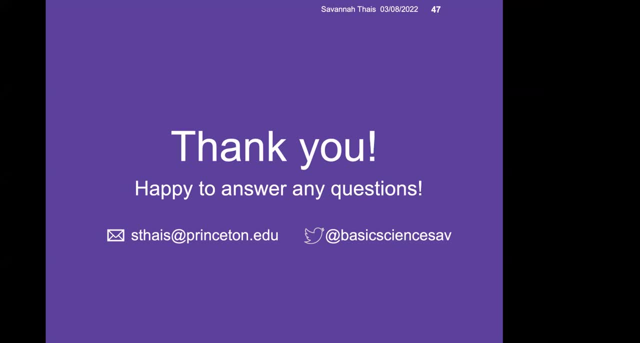 So it's all trained on simulation. right now, Monte Carlo simulation, primarily open source, but we're starting to look at also simulation from individual particle physics experiments of the Large Hadron Collider, as well as actual data from those detectors. So once we have an idea about how efficient our model actually is, we can start to use. 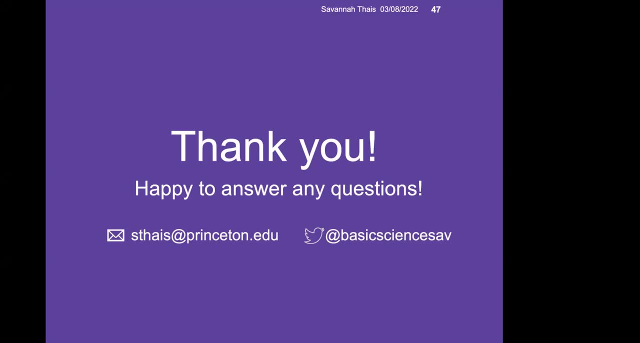 it on real data and see if it's able to translate. But right now, yeah, all of the training is Monte Carlo simulation, Thank you. We have another question from Ari. He's asking what's the best place to start if you want to get familiar with GNNs. 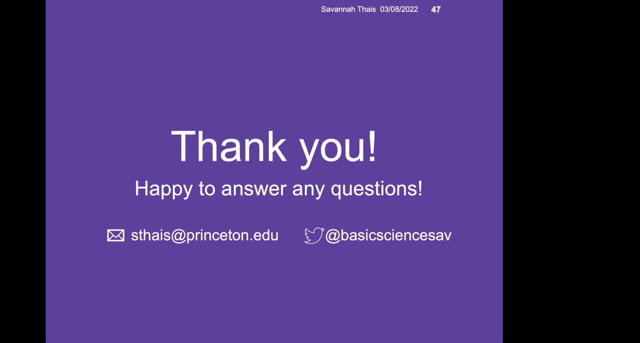 Yeah, That's a good question. So in general, I think my question is: what's the best place to start if you want to get familiar with GNNs? So Michael Bronstein had a really great talk. I'm spacing on what conference it was at right now. 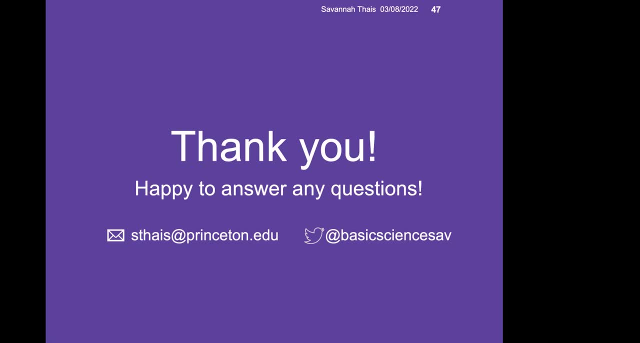 But if you Google like Michael Bronstein GNNs, it should be one of the first results. So that's a really intuitive talk, I think, with a lot of really great graphics. Then he also recently put out a book with some different collaborators. 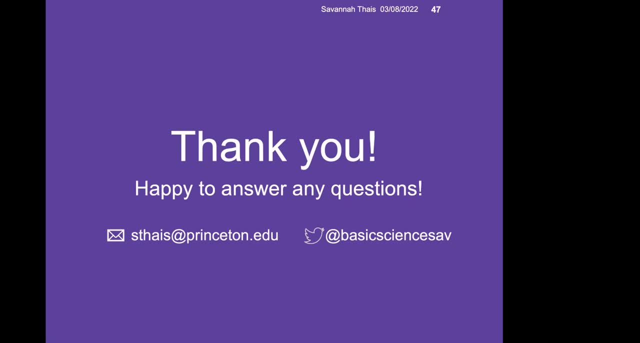 Graphs, gauges, geodesics, something like that- Geometric machine learning- graphs, gauges and geodesics- Awesome. So the link is already in the chat. And then there are some good overview papers as well that I don't necessarily remember. 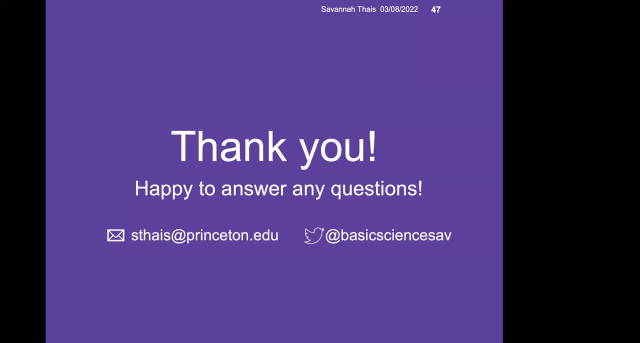 the names of right now, But I really think Michael Bronstein's material is really useful for learning. And then, If you're interested in, like particle physics, applications of GNNs, there's a great summary paper called GNNs in. 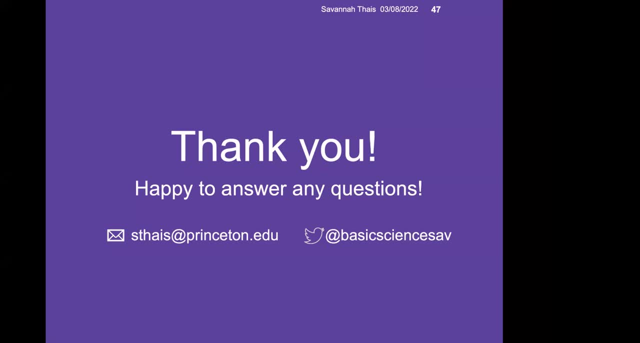 I believe it's GNNs in Particle Physics, which is written by some of my collaborators, So that's a nice summary as well, Thank you. We have a last question from Will: Are you considering using any semi-supervised approaches When transitioning from simulated to real experimental data? 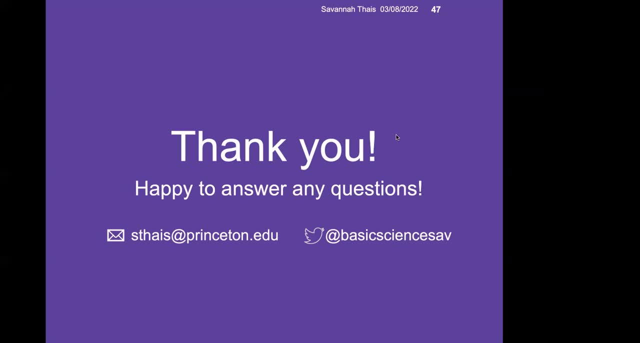 Yeah, we're definitely thinking about that. We're still really in the early stages of looking at the actual experimental data, And even going from this kind of open source detector simulation to the actual experiment simulations has required a lot of adjustments and retraining. 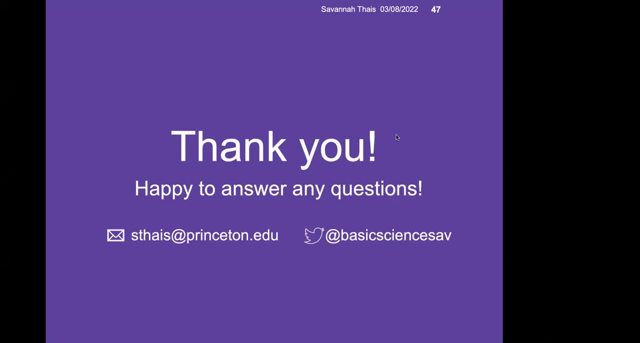 But yeah, that's definitely something we're thinking about. We're just not quite there yet. Okay, Thank you, Thank you. I think, yeah, we can close here, And thank you so much, Savannah, for doing this lecture.